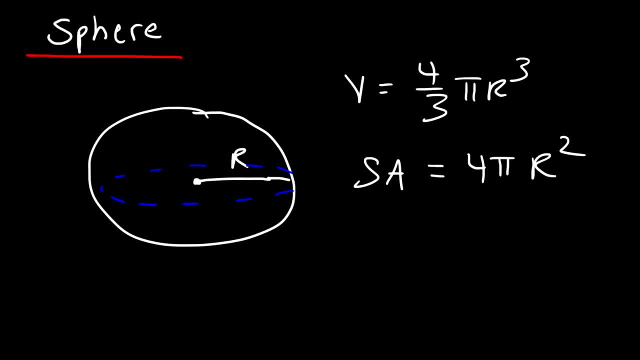 R squared where r is the radius of the sphere. So make sure you write these things down, because you need to know them if you have a test on it. Now, the next figure we need to talk about is this cylinder, And it looks like this: 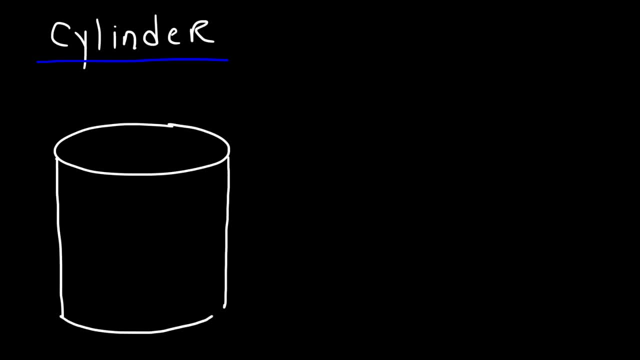 This is just a rough sketch. So this is the radius of the cylinder And here we have The height of the cylinder, The volume of the cylinder. it's the area of the base, where the base is basically a circle. The area of a circle is pi? r squared. 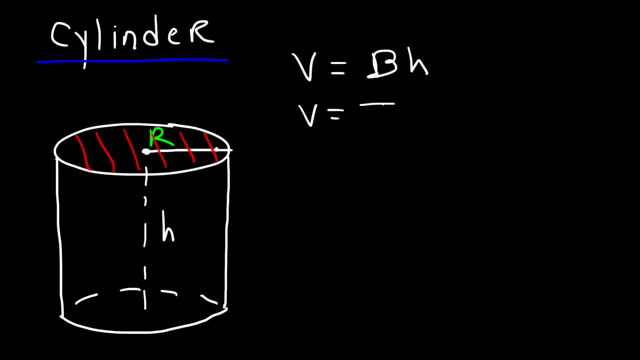 It's the area of the base times the height. So the base is pi r squared and the height is just h. So that's how you can calculate the volume of a cylinder. To calculate the total surface area of a cylinder, it's the area of the base plus the lateral surface area. 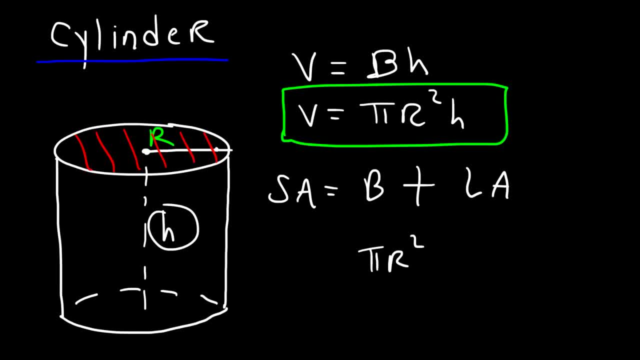 Now the area of the base is pi r squared. But notice that we have two bases, one on top and the one on the bottom, So it's 2 pi r squared. The lateral area is the product of the circumference of the circle, times the height. 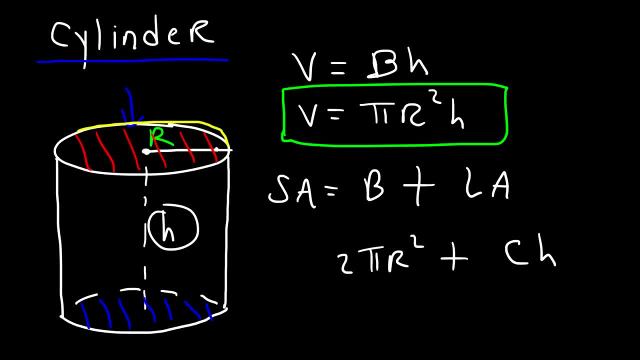 So this is The distance around the circle, is the circumference, And the circumference of a circle is 2 pi r, So you could use this equation to calculate the total surface area of a cylinder. Now, the next figure that we need to discuss is the cone. 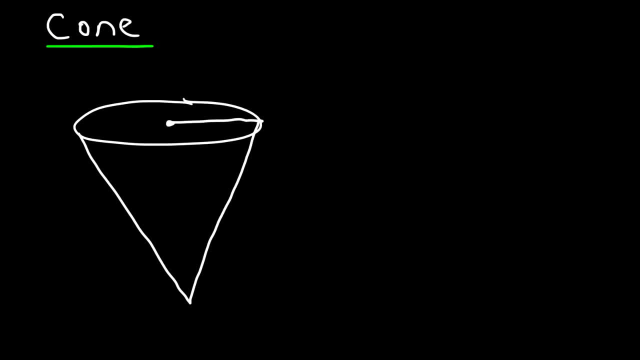 So a cone has a circumference of 2 pi r squared, a circular base and this is the radius of the cone and here this is the height of the cone. so notice that we have a right triangle. so this is R and this is H. now the hypotenuse of this right triangle is known as the slant height. 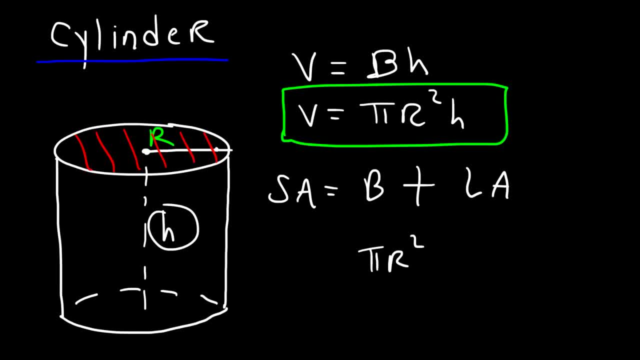 Now the area of the base is pi r squared. But notice that we have two bases, one on top and the one on the bottom, So it's 2 pi r squared. The lateral area is the product of the circumference of the circle, times the height. 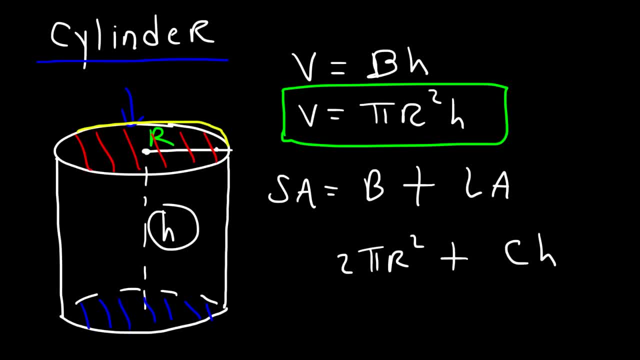 So this is the distance around the circle, is the circumference, And the circumference of a circle is 2 pi r, So you could use this equation to calculate the total surface area of a cylinder. Now, the next figure that we need to discuss is the cone. 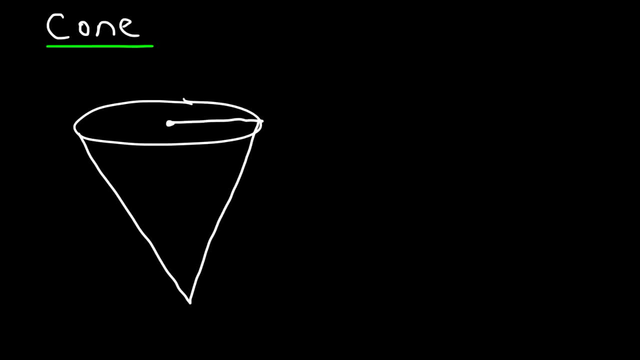 So a cone has a circumference of 2 pi r squared. It has a circular base And this is the radius of the cone And here this is the height of the cone. So notice that we have a right triangle. So this is r and this is h. 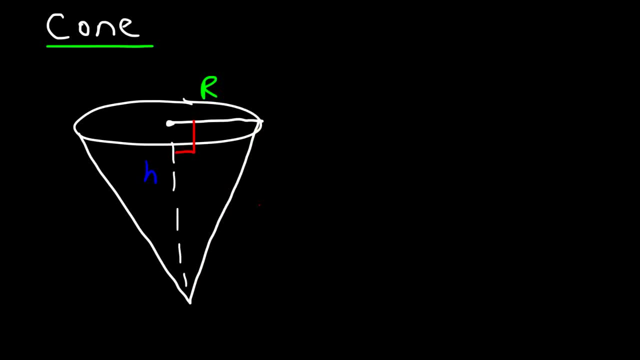 Now the hypotenuse of this right triangle is known as the slant height, which is l. The volume of a cone is 1 third of the volume of a cylinder, So it's 1 third. So it's 1 pi r squared times the height. 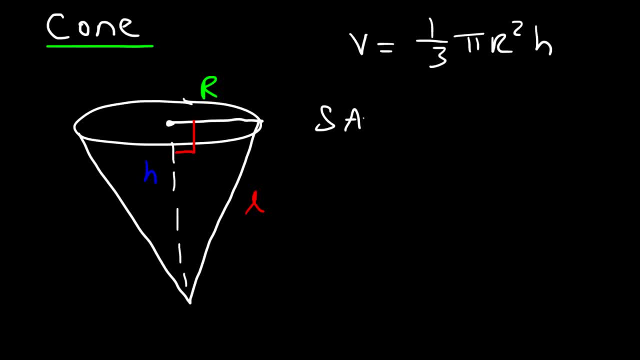 Now the surface area is the area of the base plus the lateral area, Just like before. we know, the area of the base is the area of the circle, And there's only one circle this time, not two like in the last problem. So it's 1 pi r squared as opposed to 2 pi r squared. 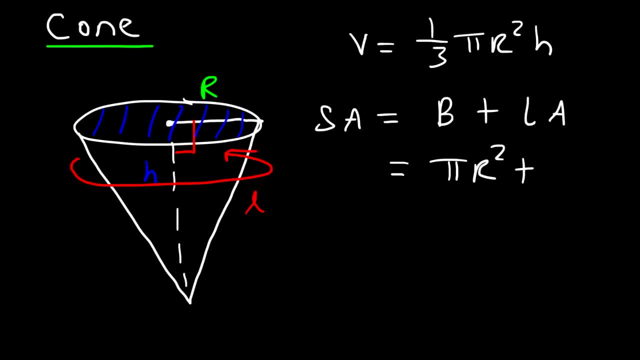 Now the lateral area is the area around the cone And it's 1 half The perimeter times the slant height. The perimeter of a circle is 2 pi r, Keep in mind. the perimeter is basically the circumference of a circle And the slant height. that's just l. 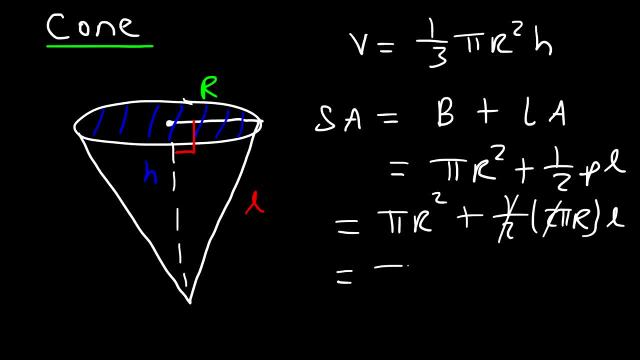 So we can cancel 1, half and 2.. Half of 2 is 1.. So the surface area of a cone works out to be this equation: It's pi r squared times pi r l. Now how can we calculate the slant height? 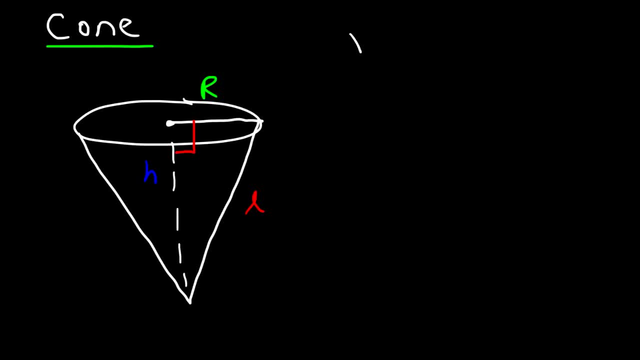 which is L. the volume of a cone is 1 third of the volume of a cylinder, so it's 1 third pi R squared times the height. now the surface area is the area of the base plus the lateral area. just like before, we know the area, the base is. 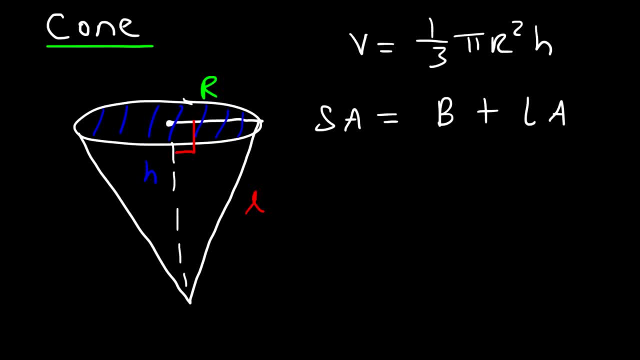 the area of the circle and there's only one circle this time, not two like in the last problem, so it's 1 pi R squared as opposed to 2 pi R squared now. the lateral area is the area around the cone and it's 1 half the perimeter times the slant height, the perimeter of a circle. 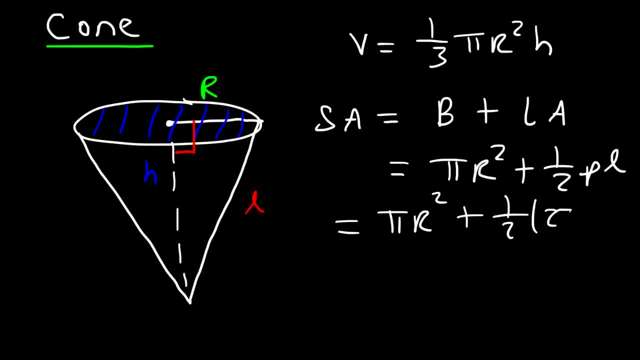 is 2 pi R. keep in mind. the perimeter is basically the circumference of a circle and the slant height. that's just L. so we can cancel 1 half and 2. half of 2 is 1. so the surface area of a cone works out to be this equation: its pi R squared times pi R L. now 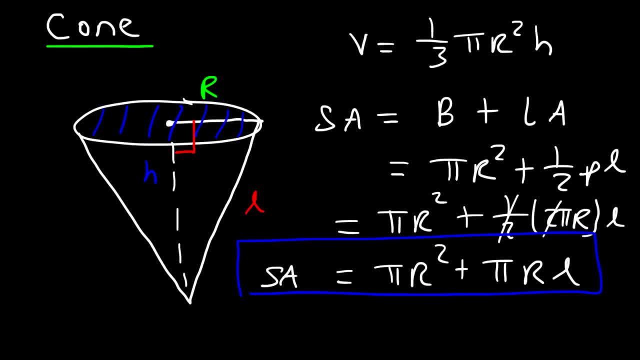 how can we calculate the slant height? the slant height L? you could find it based on the right triangle. you can use the Pythagorean theorem to get it so. for a right triangle, C squared is equal to a squared plus B squared and C is the 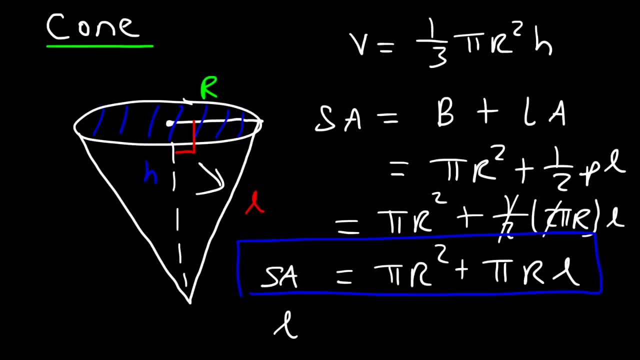 hypotenuse which correlates to the slant height. so L squared is equal to R squared plus h squared. so you can use this to calculate the slant height and once you have that you can calculate the surface area of the cone, and then you can easily. 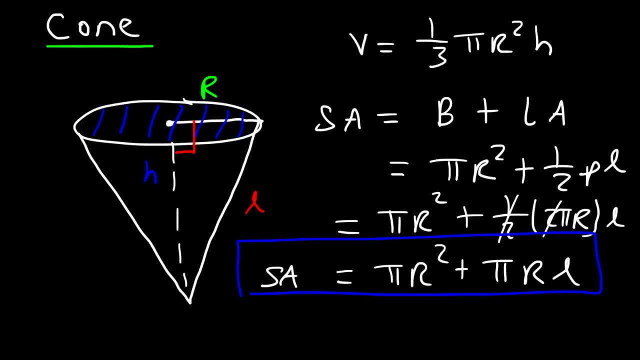 The slant height l. you can find it based on the right triangle. You can use the Pythagorean theorem to get it. So for a right triangle, c squared is equal to a squared plus b squared, And c is the hypotenuse which correlates to the slant height. 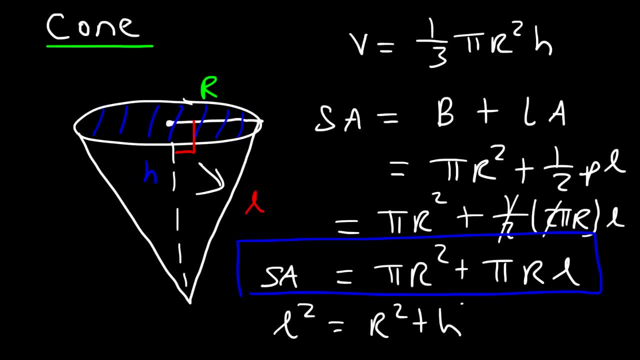 So l squared is equal to r squared plus h squared. So you can use this to calculate the slant height And once you have that you can calculate the surface area of the cone, And then you can easily calculate the volume of the cone using that formula. 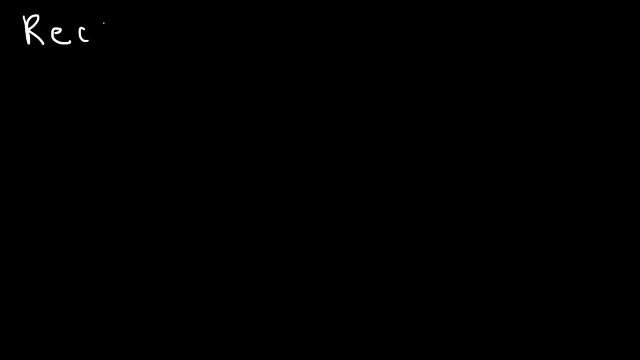 Now let's move on to the next shape, And this is the rectangular prism. So let's draw this first. So let's call this the length, the width and the height. The volume of a rectangular prism is simply the product of those three values. 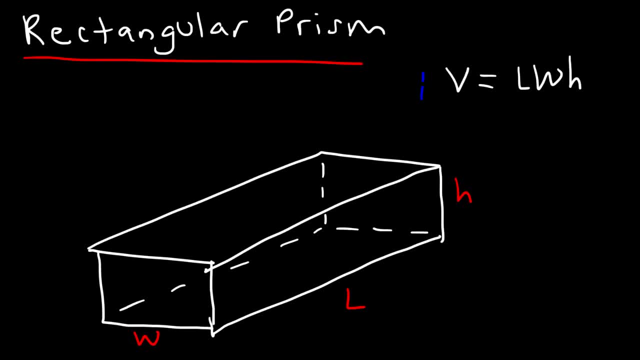 It's the length times the width times the height. Now, what about the surface area? How can we calculate that? Well, first we need to add up the area of all six faces, So let's start with the face in the front and the one in the back. 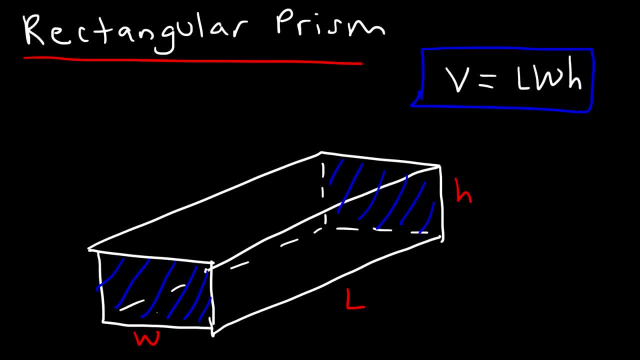 Notice that the area of each of those faces is the width times the height, Where the height is h And it's two of them, so it's going to be 2w. So that's the area of the front and the back. 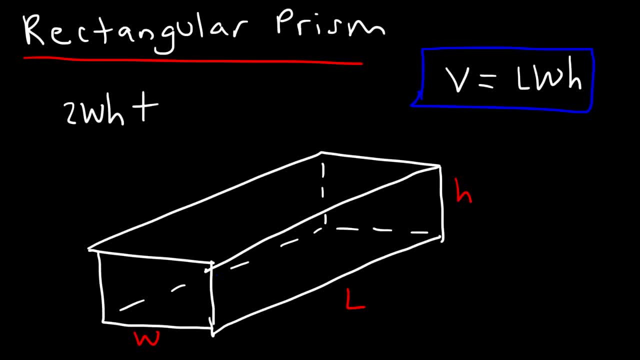 Now let's calculate the area of the sides, So let's say the front side and the back side or the side on the left. So notice that it has the length l and the height h, So the area of those two sides is going to be lh but times 2.. 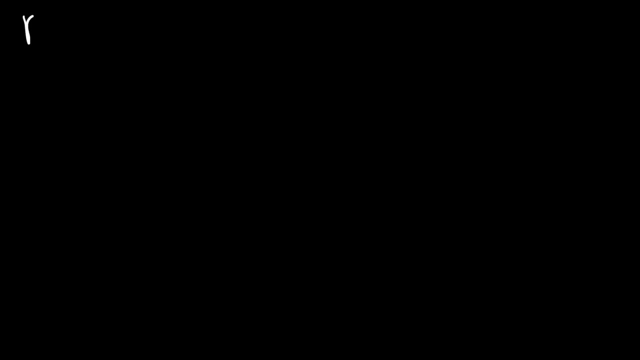 calculate the volume of a cone using that formula. now let's move on to the next shape, and this is the rectangular prism. so let's draw this first. so let's call this the length, the width and the height. the volume of a rectangular prism is simply the product of those three values, is the length times the. 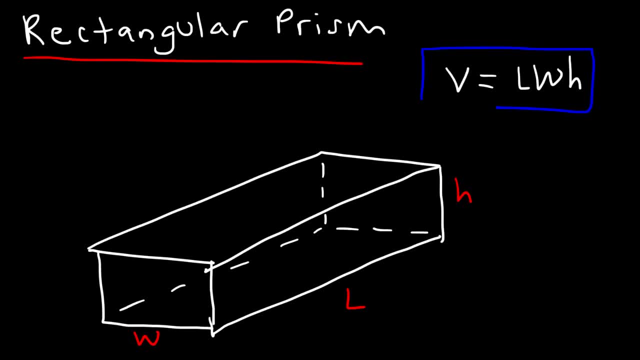 width times the height. now, what about the surface area? how can we calculate that? well, first we need to add up the area of all six faces. so let's start with the face in the front and the one in the back. notice that the area of each of 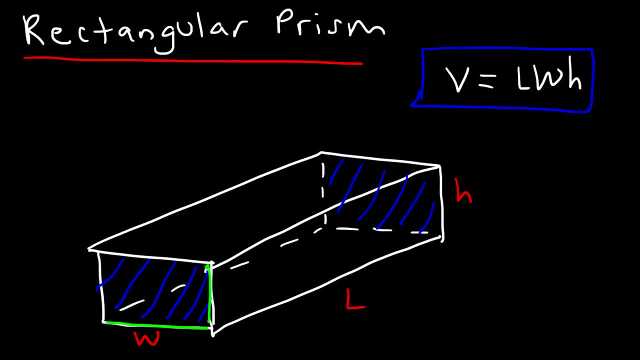 those faces is the width times the height, where the height is h and it's two of them, so it's going to be 2wh. so that's the area of the front and the back. now let's calculate the area of the sides, so let's say the front side and the back side, or the side on the left. so 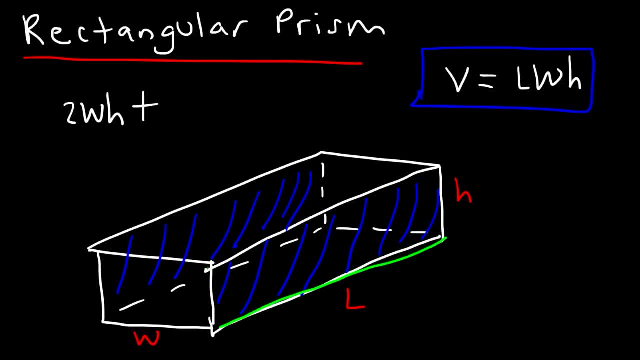 notice that it has the length l and the height h, so the area of those two sides is going to be lh, but times 2 or 2 lh. and then we need to calculate the area of the top face and the bottom face, so it's the width times the length and then times 2, so that's going to be 2 lw. so 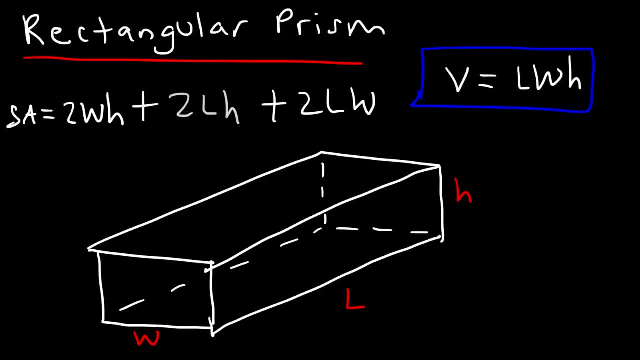 this will give you the surface area of a rectangular prism. now, sometimes you may need to calculate the length of the diagonal. let's call it d. if you ever need to do that, here's the formula you need. d is equal to the square root of l, squared plus w. 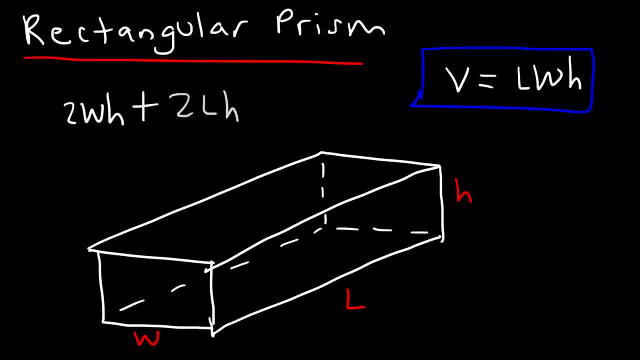 Or 2lh, And then we need to calculate the area of the top face and the bottom face. So it's the width times the length and then times 2.. So that's going to be 2lw. So this will give you the surface area of a rectangular prism. 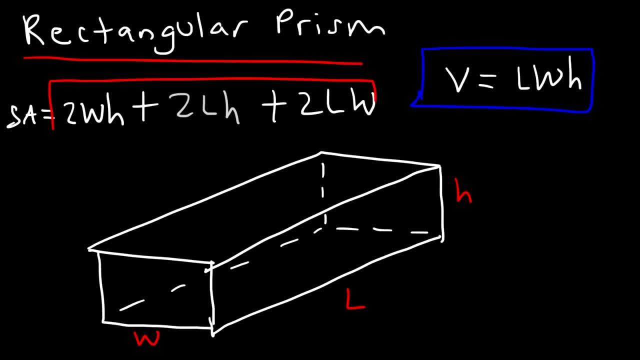 Now, sometimes you may need to calculate the length of the diagonal. Let's call it d. If you ever need to do that, here's the formula you need. d is equal to the square root of l, squared plus w squared plus h squared. 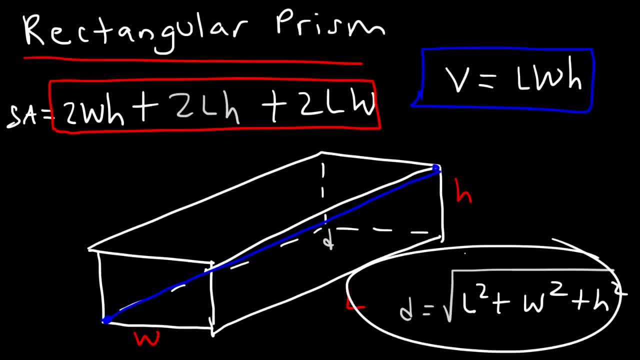 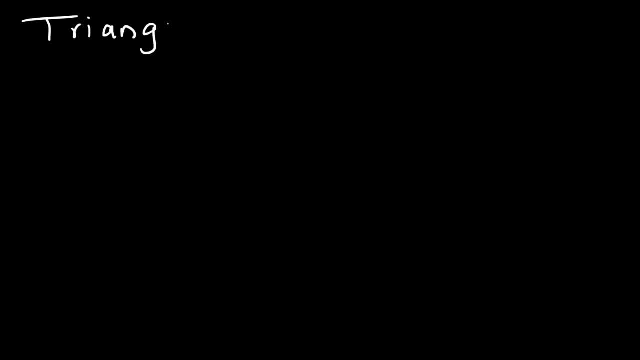 And so that's how you can calculate the length of the diagonal of a rectangular prism. Now the next shape we need to talk about is the triangular prism. Now, there's multiple ways in which we can draw this figure, So one way we can draw it is like this: 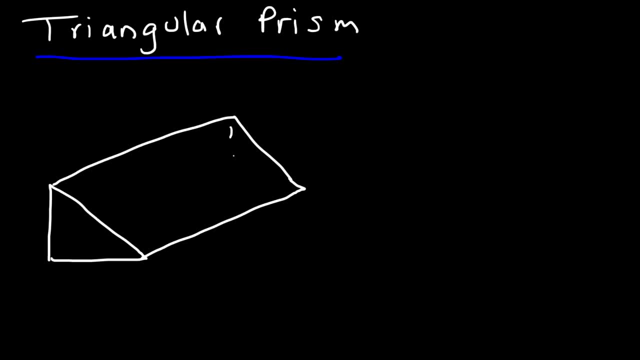 The base could be a right triangle, It can be an equilateral triangle, So it could be many things. So, in this example, let's say that this is the base, This is the height, And this is the height of the prism itself, which I'm going to distinguish it from this h by using capital H. 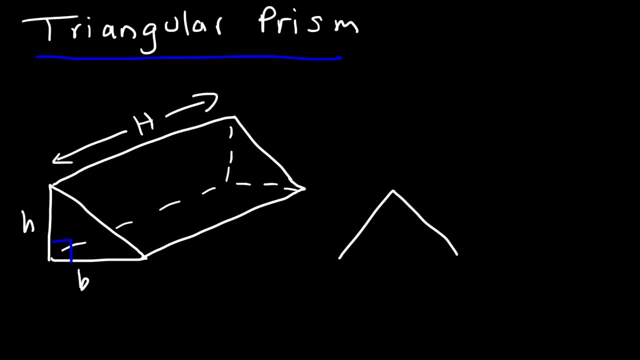 Now we can also draw a triangular prism like this, So this would still be h In this case. this is the base And this would be the height of the triangle. Now, the volume of a triangular prism is the base times the height. 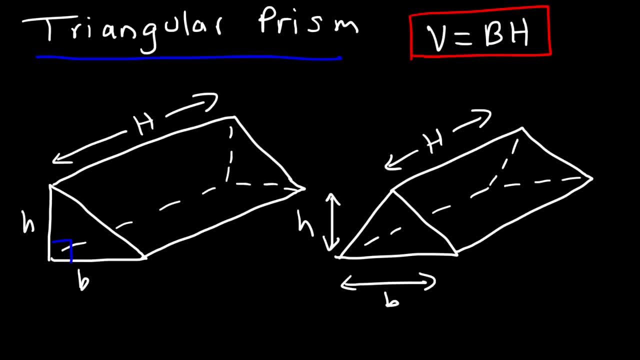 Capital B is the area of the base, And the area of the base can vary. In this case, it's simply the area of a triangle. For a right triangle, you can calculate the area using this formula: It's one half base times height. 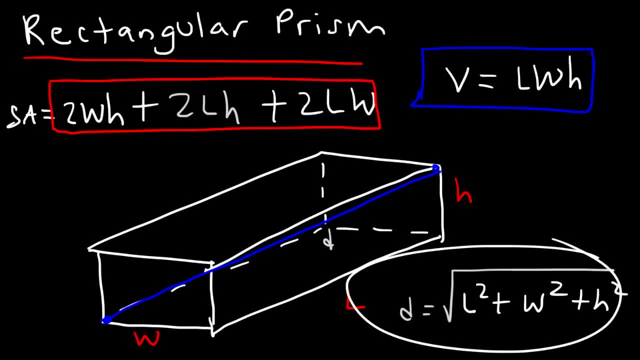 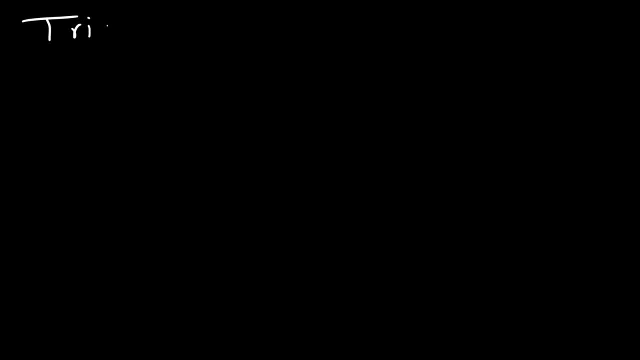 squared plus h squared, and so that's how you can calculate the length of the diagonal of a rectangular prism. now the next shape we need to talk about is the triangular prism. now there's multiple ways in which we can draw this figure, so one way you can draw it is like this: the base could be a right triangle, it can be. 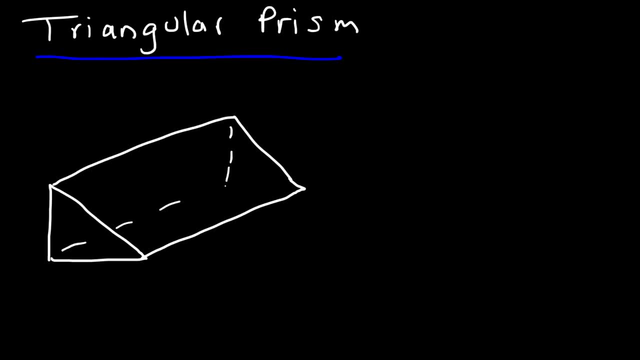 an equilateral triangle, so it could be many things. so in this example, let's say that this is the base, this is the height, and this is the bottom, and this is the height and this is the height of the prism itself, which I'm going to distinguish it from this H by using capital H. now we can also draw a. 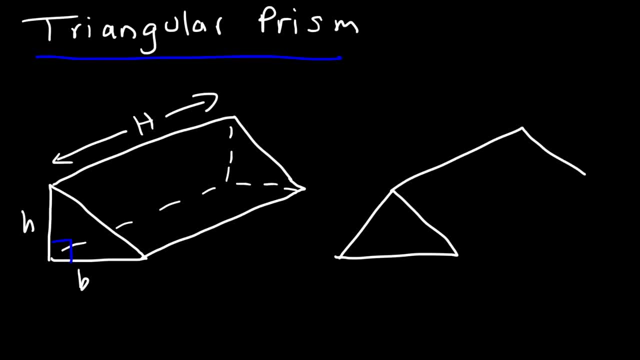 triangle, a triangular prism, excuse me, like this. so this would still be H in this case. this is the base and this would still be the height of the triangle. now, the volume of a triangular prism is the base times the height capital. B is the area of the base and the area of the base can. 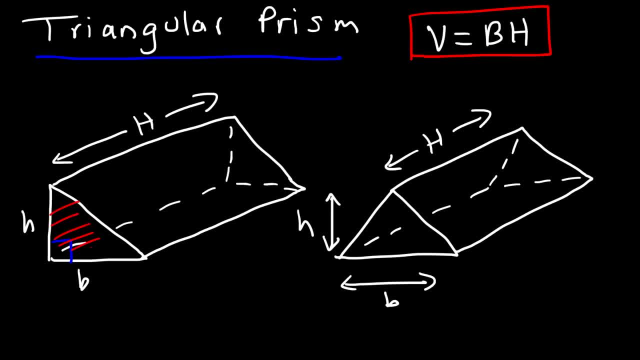 vary. in this case it's simply the area of a triangle. for right triangle, you can calculate the area using this formula: it's one-half base times height, so this would equal capital B. now let's say, if you have an equal triangle where all three sides are the same, The area is the square root of 3. 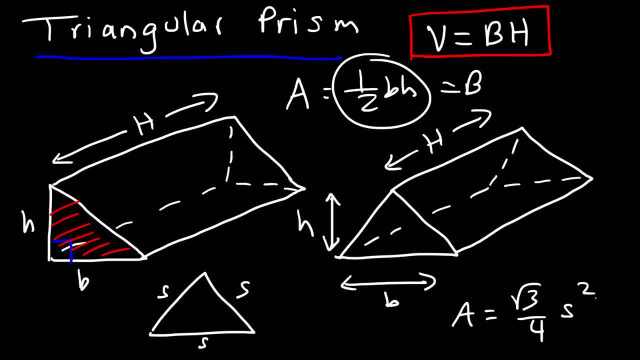 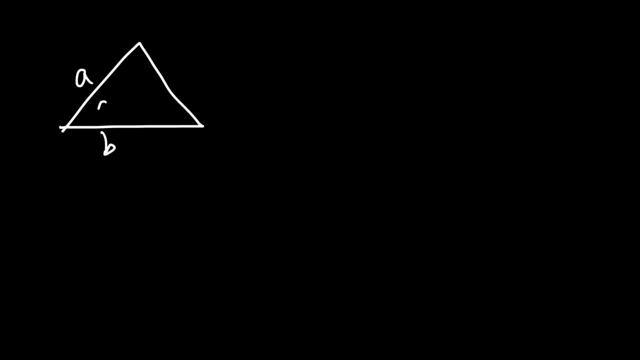 over 4 times s squared. Now, let's say, if you had a triangle where you have two sides and included angle, the area is 1 half AB sine of angle C. Now if you have a triangle like this, let's say, if you know the base and the height, you could 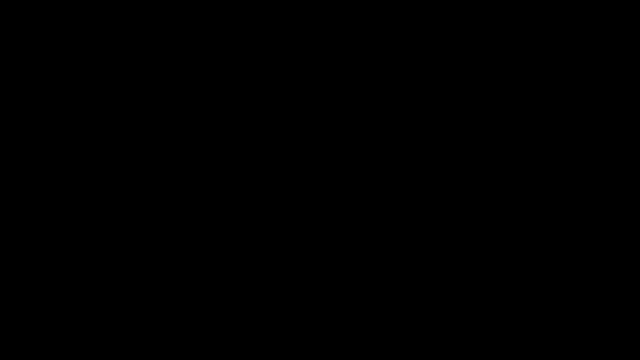 simply use: a is equal to 1 half BH. Now sometimes you may have a triangle where you're given all three sides and let's say all three sides are different. If you need to calculate the area of this triangle, you need to calculate s first. 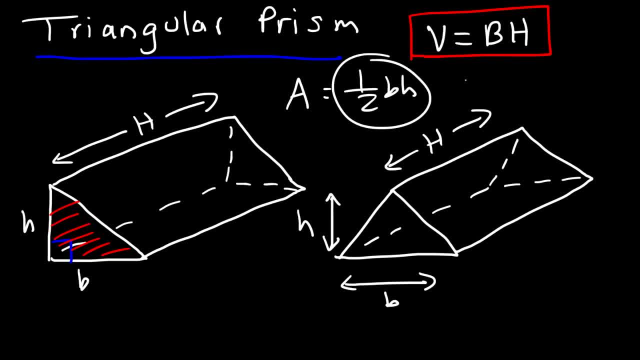 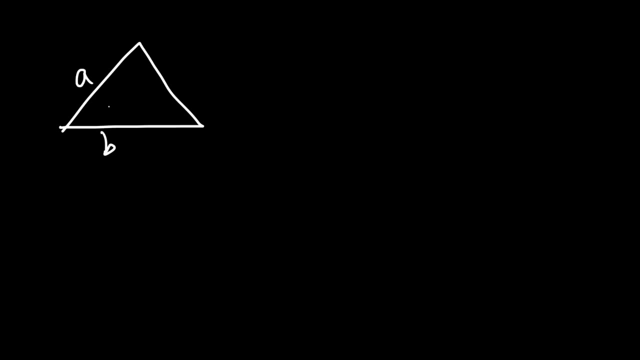 So this would equal capital B. Now let's say if you have an equilateral triangle where all three sides are the same, The area is the square root of 3 over 4 times S squared. Now let's say if you had a triangle where you have two sides and the included angle 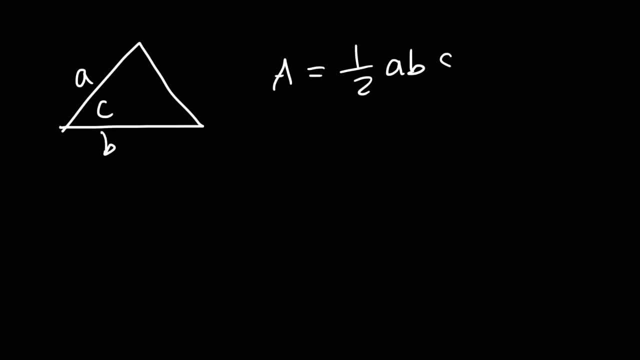 The area is one half AB, Sine of angle C. Now if you have a triangle like this- let's say, if you know the base and the height, You could simply use: A is equal to one half BH. Now, sometimes you may have a triangle where you're given all three sides. 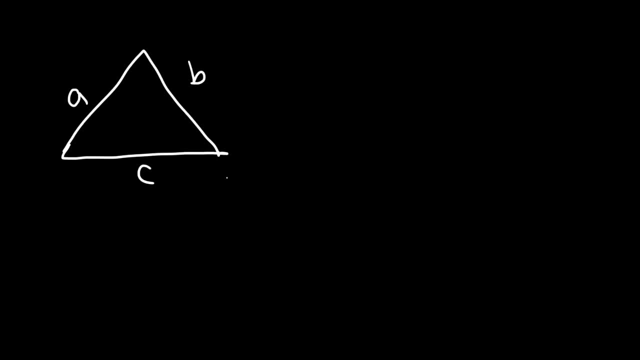 And let's say all three sides are different. If you need to calculate the area of this triangle, you need to calculate S first, Which is one half of the perimeter of the triangle, And then you can use Huron's formula to calculate the area. 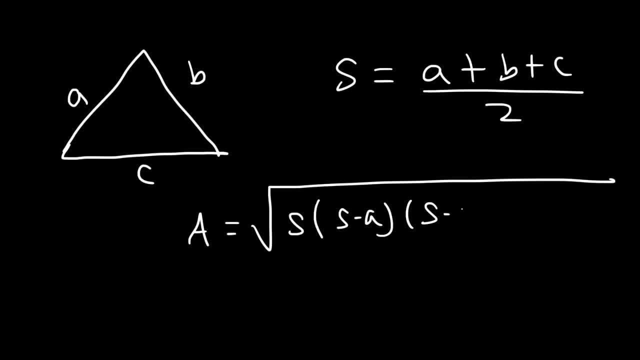 It's S times S minus A, times S minus B, times S minus C, And that result is all within the square root. So that's another way in which you can calculate the area of the triangle. So once you find the area, you can replace B with it. 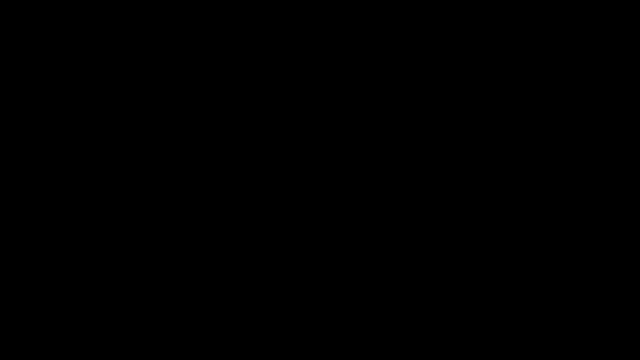 And then you can calculate the volume of a triangular prism. Now, sometimes you might see a triangular prism drawn this way, And so you're still dealing with the same type of shape. This is the height of the prism. This is the base of the triangle. 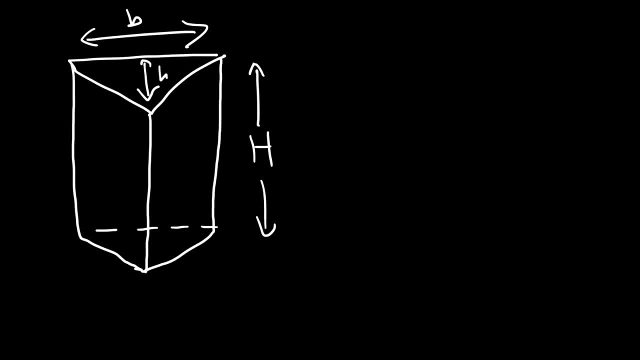 And you could say: this is the height of the triangle. Now let's go back to this figure. How can we calculate the surface area Of a triangular prism? Now, keep in mind, the formula can vary. This is the base, This is the height. 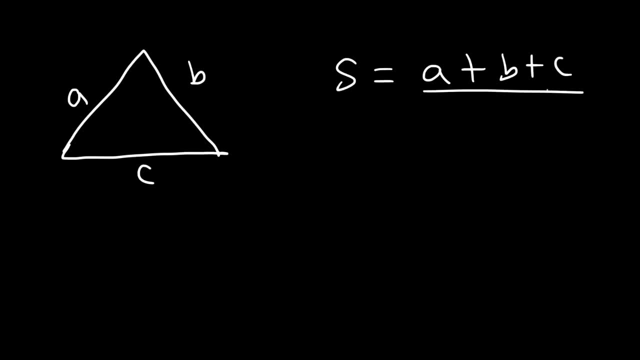 which is 1 half of the perimeter of the triangle, and then you can use Huron's formula to calculate the area. It's s times s minus a, times s minus b, times s minus c, and that result is all within the square root. So that's another way in which you can calculate the area of the. 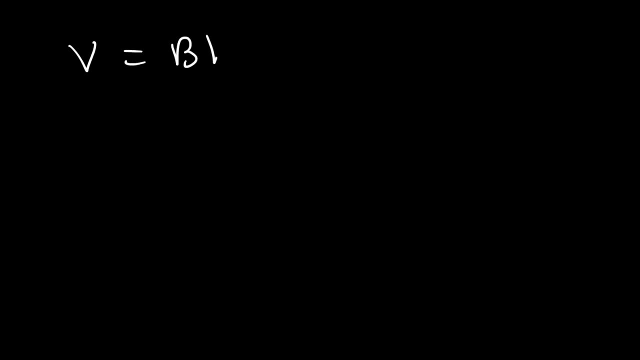 triangle. So once you find the area, you can replace b with it, and then you can calculate the volume of a triangular prism. Now, sometimes you might see a triangular prism drawn this way, And so you're still dealing with the same type of shape. This is the height of 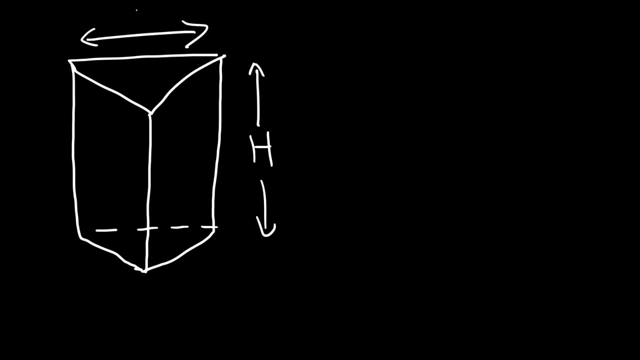 the prism. this is the base of the triangle and you can say this is the height of the triangle. Now let's go back to this figure. How can we calculate the surface area of a triangular prism? How can we calculate the surface area of a triangular prism? 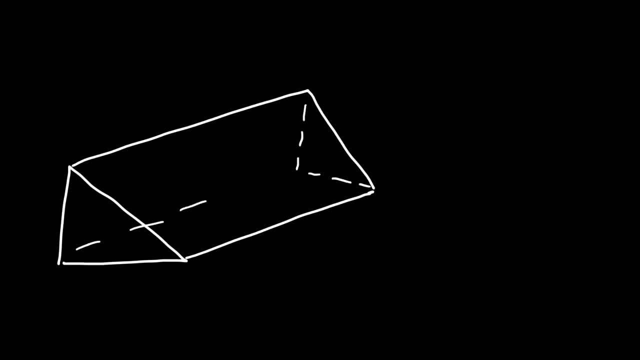 Now, keep in mind, the formula can vary. This is the base, this is the height and this is the height of the prism. The general formula is this: The surface area is the area of the base plus the lateral area. Now the area of the base is going to. 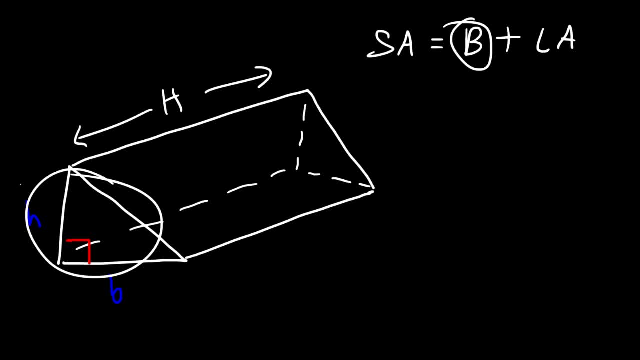 change depending on what type of triangle you have. Is it the right triangle? do you have all three sides? are the three sides different at the same, and so this can vary. but for this particular triangle- I'm just going to give an example- the area, the base, is going to be the area of the triangle, which is 1 half base times. 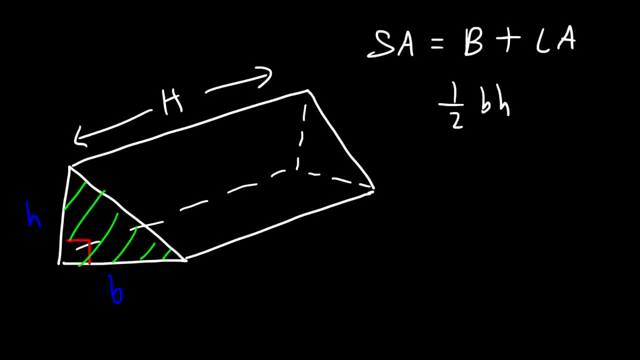 height. now there's two of them. we have the triangle on the left and on the right, so we got to multiply that by 2. so for this particular example, capital B is 2 times 1 half BH. now the lateral area is going to be the area of the other. 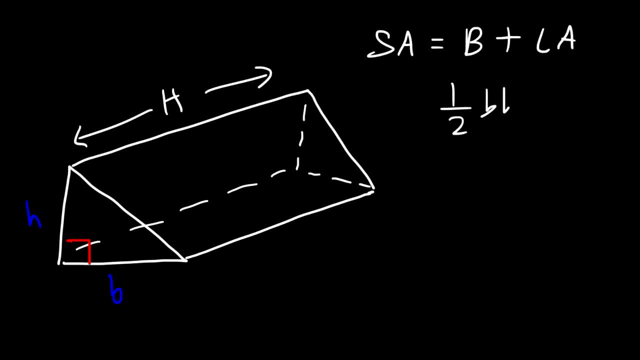 three sides, or three faces, rather, let's call the third side of the triangle L. so since we have a right triangle, L squared is equal to B squared plus H squared. so if we wish to change that, we can do that by multiplying the two sides of the triangle by the. 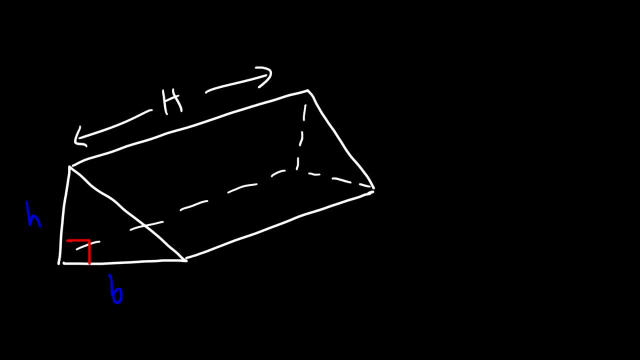 And this is the height of the prism. The general formula is this: The surface area is the area of the base plus the lateral area. Now the area of the base is going to change depending on what type of triangle you have. Is it a right triangle? 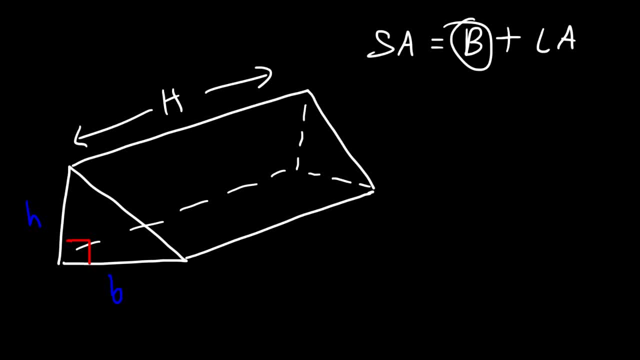 Do you have all three sides? Are the three sides different? The same, And so this can vary. But for this particular triangle, I'm just going to give an example: The area of the base is going to be the area of the triangle. 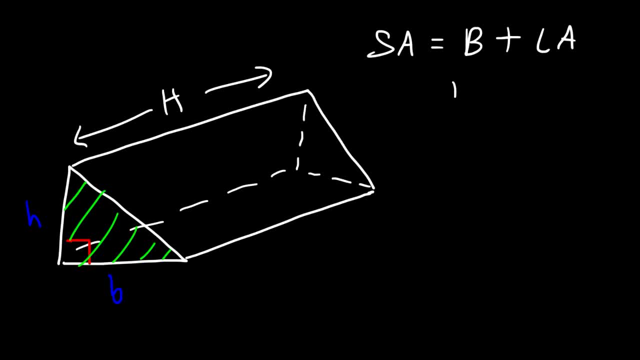 Which is one half base times height. Now there's two of them. We have the triangle on the left and on the right, So we've got to multiply that by two. So for this particular example, capital B is two times one half BH. 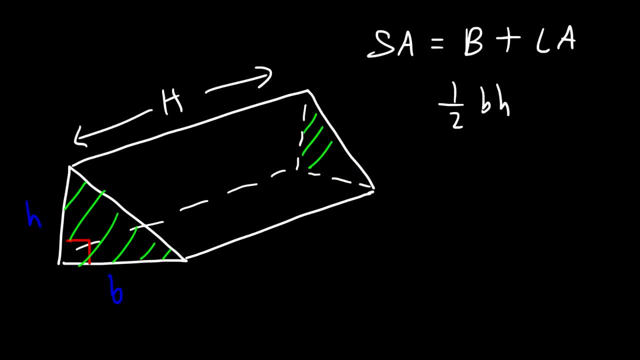 Now the lateral area is going to be the area of the other three sides, Or three faces, rather. Let's call the third side of the triangle L. So since we have a right triangle, L squared is equal to B squared plus H squared. 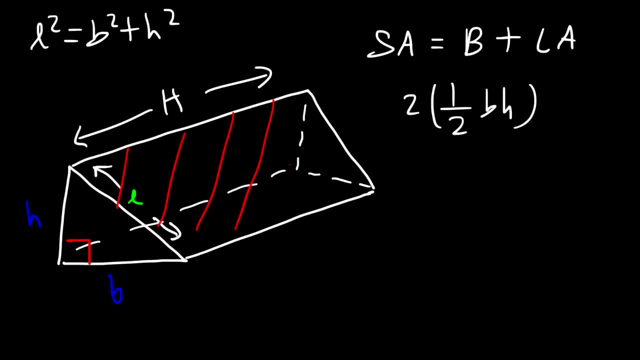 So if we wish to calculate the area of this face right here, the top face, it's going to be L times the height of the prism, So that's LH. Now let's say if we want to calculate the area of the face in the back, 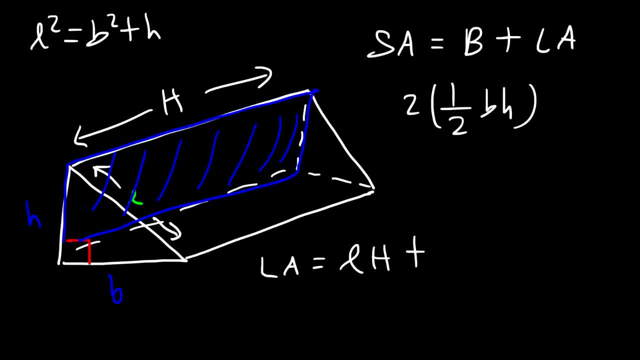 Which is this face right here It has a height H and another side length, which is lowercase h. So it's going to be H times H And then, if we want to calculate the area of the bottom face, it still has a height H, but a width of lowercase b. 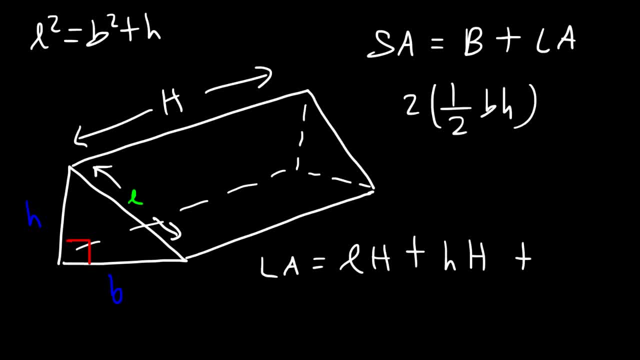 So it's going to be BH. So notice that it's basically the perimeter of the triangle, Which is the sum of those three sides- H, L and B- times the height of the prism. If you factor out capital H, you could see that P is equal to L plus H plus B. 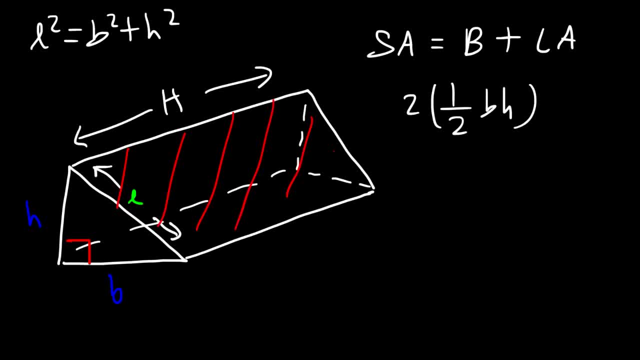 right triangle, L squared plus H squared. so if we wish to calculate the area of this face right here, the top face, it's going to be L times the height of the prism. so that's LH. now, let's say, if we want to calculate the area of the face in the back, which is this face right, 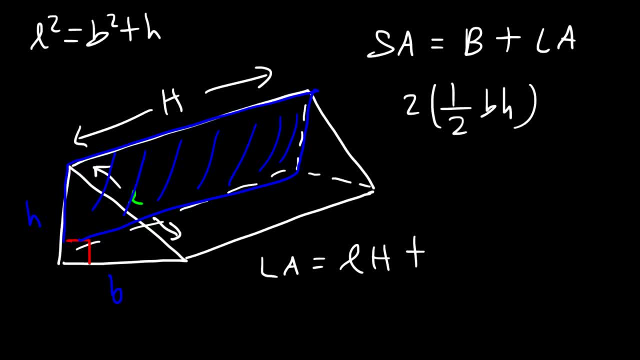 here it has a height H and another side length, which is lowercase H, so it's going to be H times H. and then, if we want to calculate the area of the bottom face, it still has a height H but a width of lowercase B, so it's going to be BH. so notice that it's. 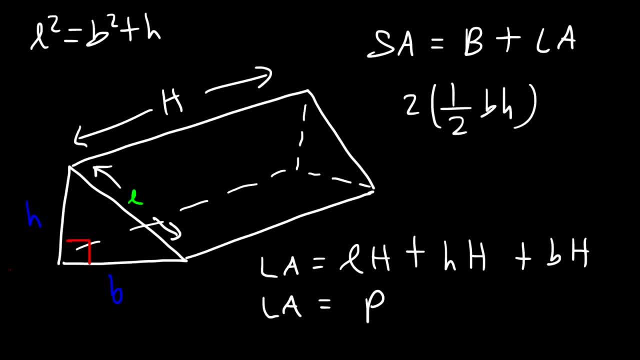 basically, the perimeter of this triangle is going to be the perimeter of the the triangle, which is the sum of those three sides- H, L and B- times the height of the prism. If you factor out capital H, you could see that P is equal to L plus H plus B. 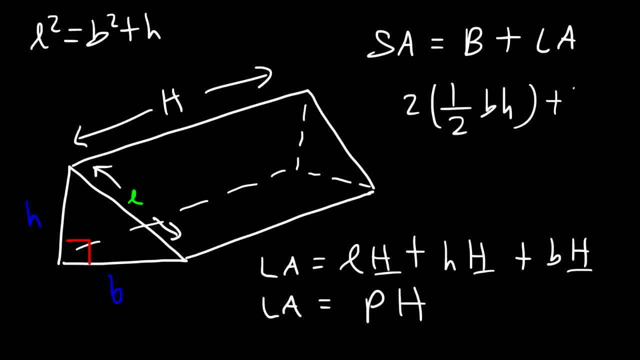 So for this particular example, the lateral area is capital H times L plus H plus B, and I'm running out of space. So thus we have: the surface area is B times H plus L plus H plus B times the height of the prism. 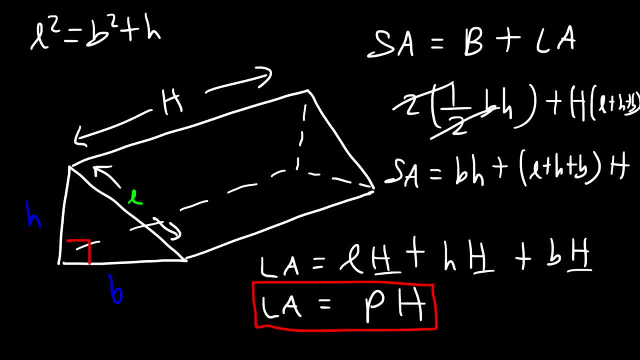 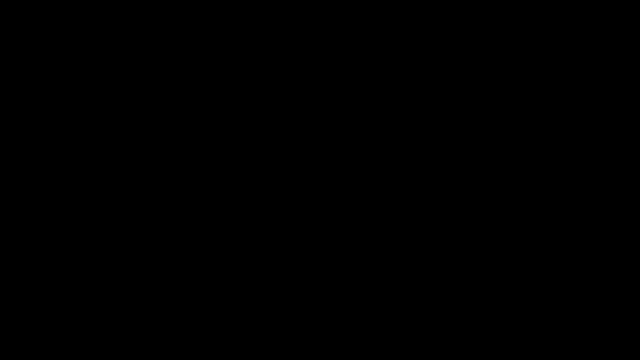 So make sure you know this: The lateral area is going to be the perimeter times the height, And so this is the surface area for this particular type of triangular prism, And you can use the general equation for all types of triangular prisms. Now there's one more shape that I want to cover, and it's the square pyramid. 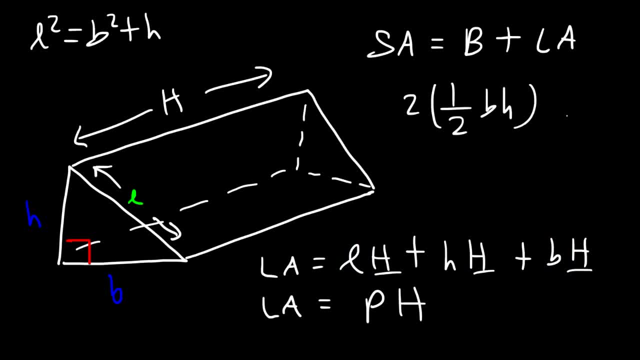 So for this particular example, the lateral area is capital H, Capital H times L plus H plus B, And I'm running out of space. So thus we have the surface area is B times H plus L plus H plus B times the height of the prism. 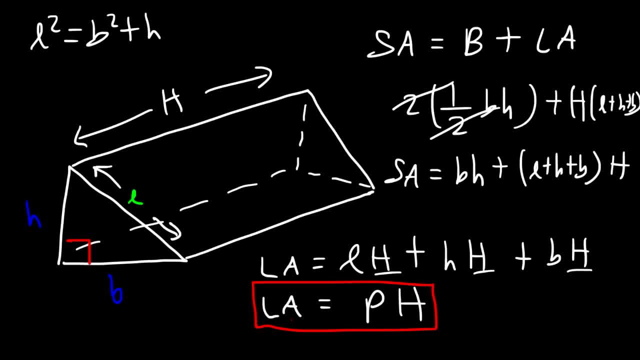 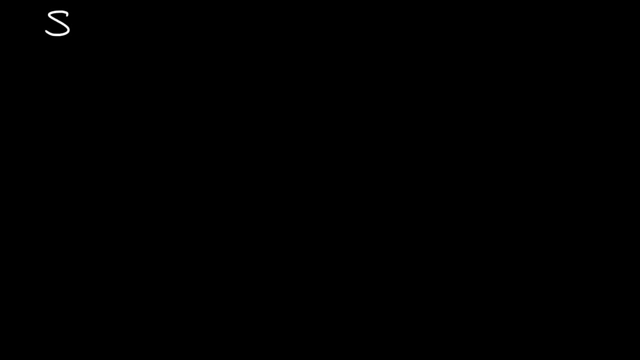 So make sure you know this: The lateral area is going to be the perimeter times the height, And so this is the surface area for this particular type of triangular prism, And you can use the general equation for all types of triangular prisms. Now there's one more shape that I want to cover. 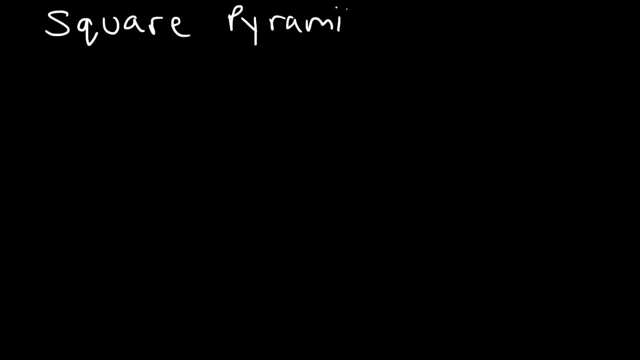 And it's the square pyramid, So it's a pyramid with the base of a square. So I'm going to draw it like this, So let's call this B, And this is going to be B as well. That's the length of the base. 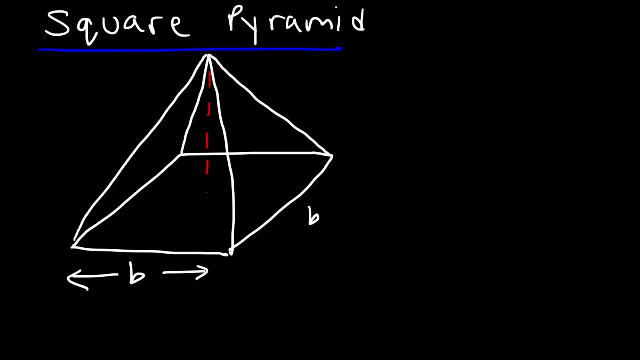 And here we have the height of the pyramid, which I'm going to call H, And this part here, that's half of B. If this whole thing is B, and this is the center, then this part here is going to be B over 2.. 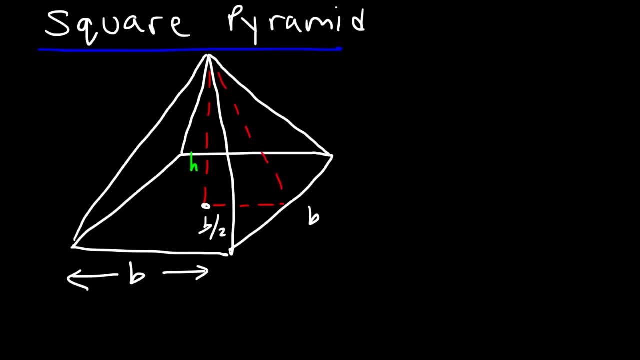 And then this part is the slant height, which we can call L, And this is the right triangle. Now the volume of a square base pyramid is going to be 1 third times the area of the base, times the height of the pyramid. 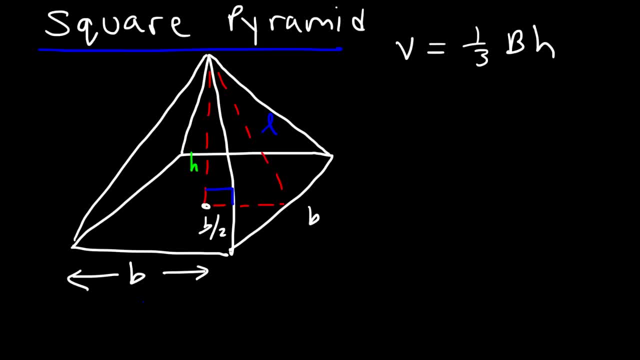 Now, the base is a square And the area of a square is length times width, or B times B, which is B squared. So capital B is equal to lower case B squared. That's the area of the base or the area of the square. 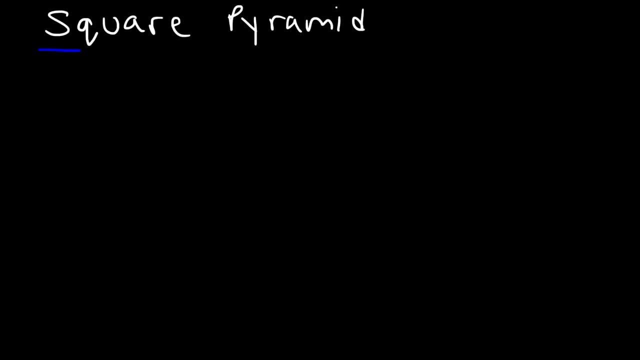 So it's a pyramid with the base of a square, So I'm going to draw it like this. So let's call this B, and this is going to be B as well. That's the length of the base, And here we have the height of the pyramid, which I'm going to call H, and this part here. 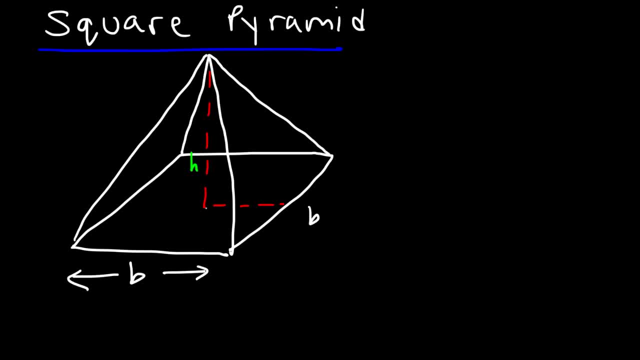 that's half of B. If this whole thing is B and this is the center, then this part here is going to be B over 2.. And then this part is the slant height, which we can call L, and this is the right triangle. 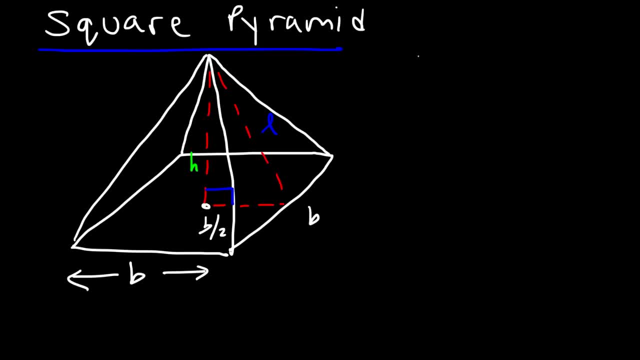 Now the volume of a square base pyramid is going to be one-third times the area of the base times the height of the pyramid. Now the base is a square and the area of a square is 1. Length times width, or B times B, which is B squared. 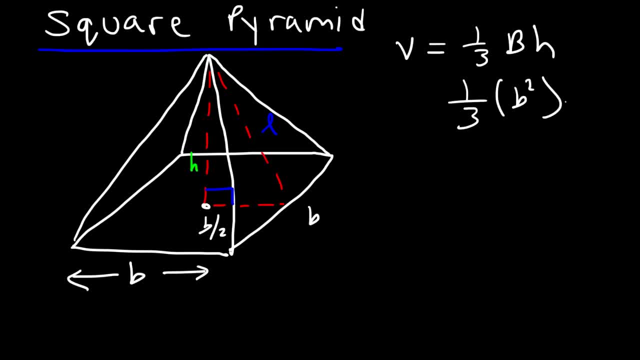 So capital B is equal to lower case B squared, That's the area of the base or the area of the square, So times the height. So therefore the volume of a square base pyramid is one-third B squared times H, where lower case B is the length of the square on the bottom. 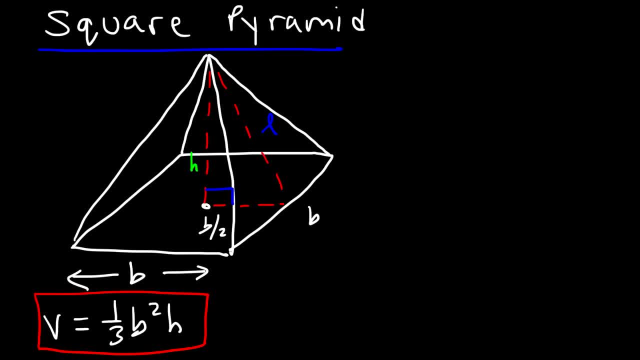 Now, what about the surface area of a square base pyramid? Okay, Well, we can use the general form for the surface area of any 3D shape: It's the area of the base plus the lateral area. Now, we know the area of the base is B squared, but what's the lateral area? 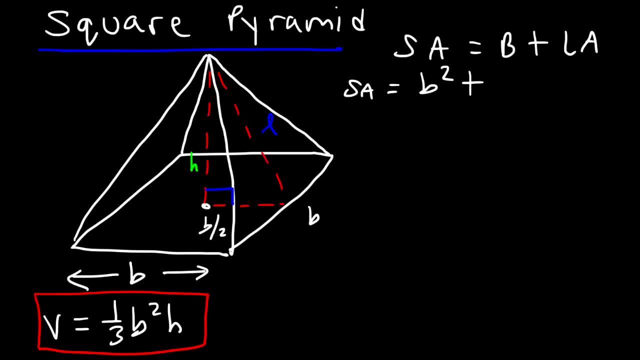 Well notice that there's four faces of four triangular faces, with one square face on the bottom. So I'm going to draw one of those four triangular faces. The height of that triangular face is the slant height, which is L, And it has a base B. 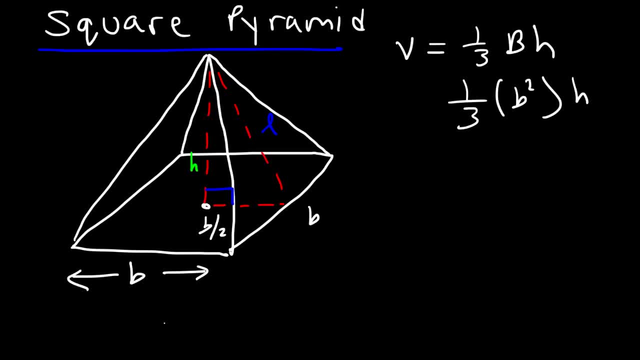 So times the height. So therefore, the volume of a square base pyramid is 1 third B squared times H, Where lower case B is the length of the square on the bottom. Now, what about the surface area of a square base pyramid? Well, we can use the general form. 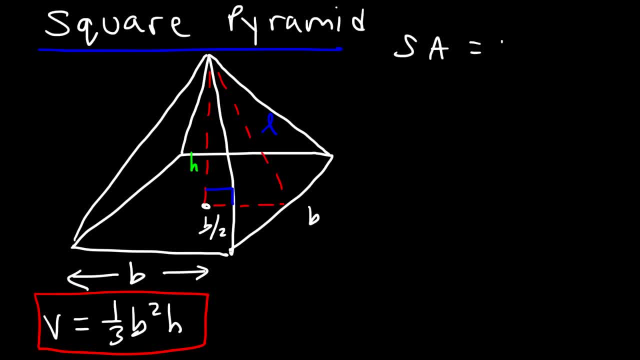 for the surface area of any 3D shape. It's the area of the base plus the lateral area. Now, we know the area of the base is B squared, But what's the lateral area? Well, notice that there's four faces of four triangular faces. 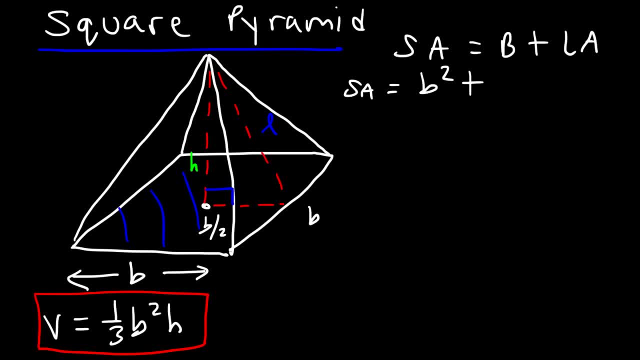 with one square face on the bottom. So I'm going to draw one of those four triangular faces. The height of that triangular face is the slant height, which is L, And it has a base B. Now we know that the area of a triangle 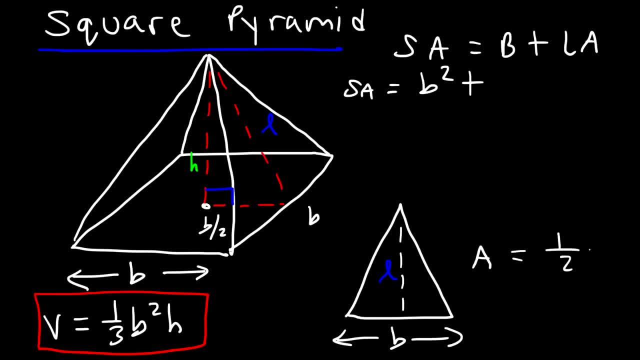 is 1 half base times height. The base B is the same, But the height is no longer H, It's the slant height, L. Now notice that we have four of those triangular faces, So this is one of them. 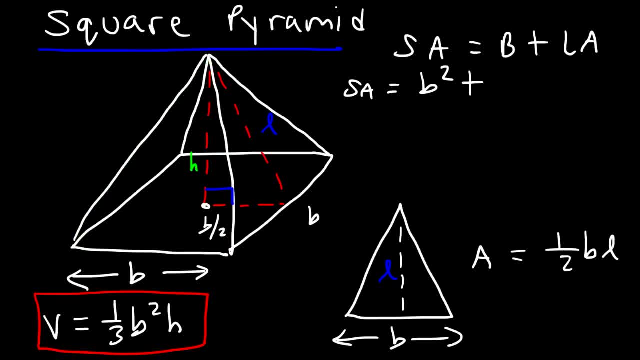 Here's the second one, That's the one in the front, Then we have the one on the left side, That's the third one, And then there's the one in the back, the fourth one. So the lateral area is going to be this times 4.. 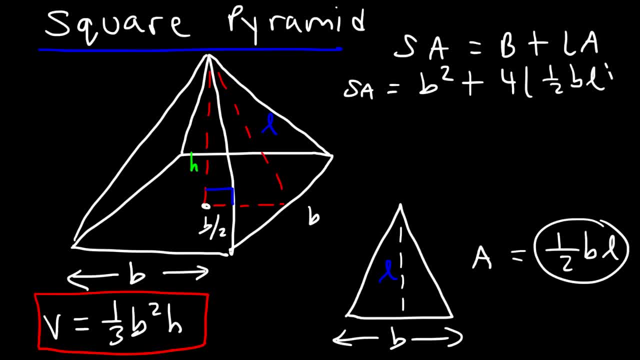 So it's 4 times 1 half B L And 4 times 1 half, or 4 divided by 2, is 2.. So this is the surface area of a square base pyramid. It's B squared plus 2 B L. 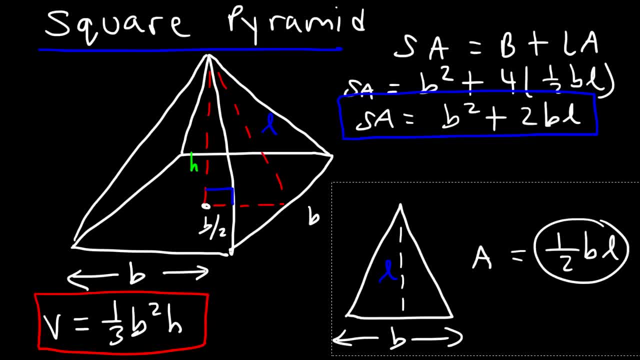 where L is the slant height. Now, how can we calculate the slant height? Let's focus on this right triangle. And so C squared is equal to A squared plus B squared, according to the Pythagorean theorem, But C is the slant height. 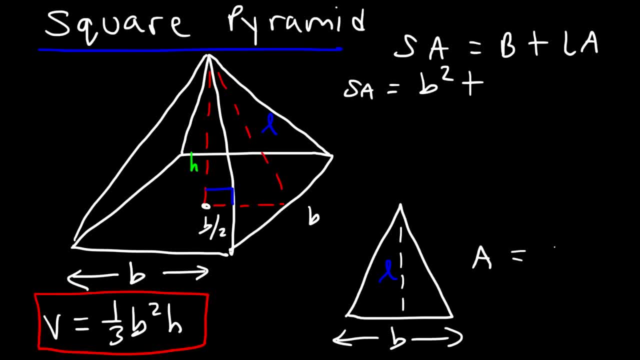 Now we know that the area of a triangle is one-half base times height. The base B is the same, but the height is no longer H, It's the slant height, L. Now notice that we have four of those triangular faces. 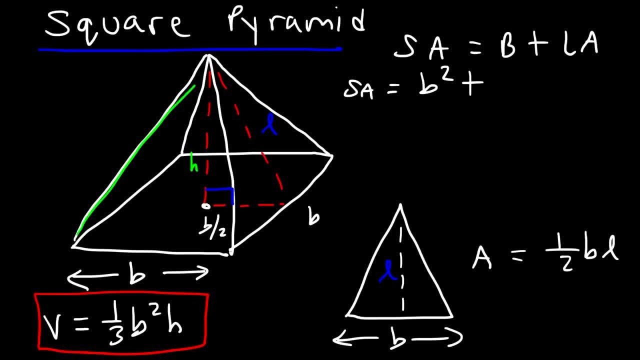 So this is one of them. Here's the second one, That's the one in the front, Then we have the one on the left side. That's the third one, And then there's the one in the back, the fourth one. 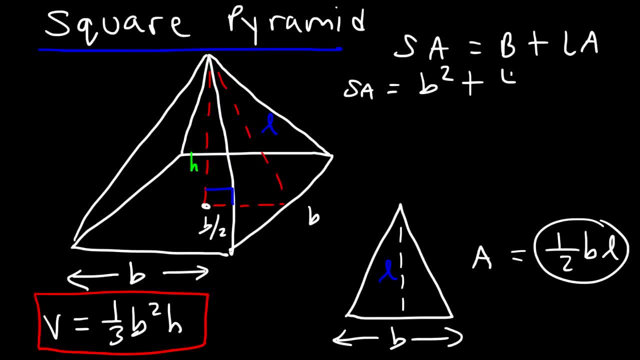 So the lateral area is going to be this times four. So it's four times one-half B? L And four times a half, or four divided by two is two. So this is the surface area of a square base pyramid. 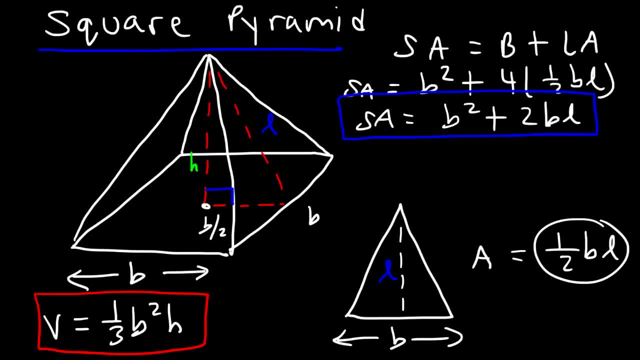 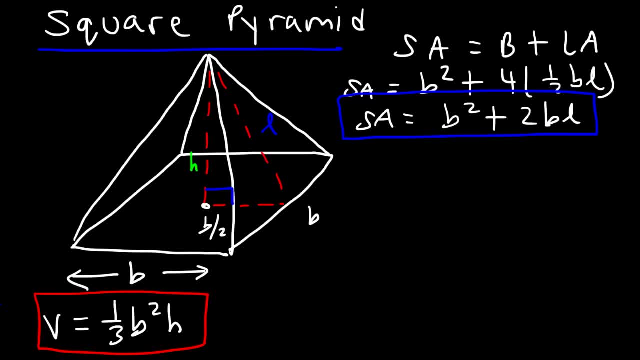 Now, how can we calculate the slant height? Let's focus on this right triangle. And so C squared is equal to A squared plus B squared, according to the Pythagorean theorem, But C is the slant height, A, which we'll call B over two. 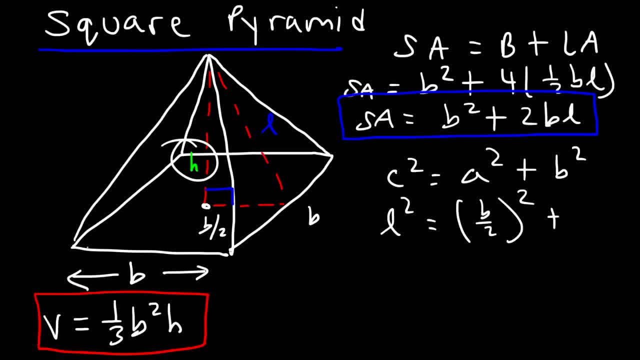 And let's square that, And then B will be H. So if you need to find the volume, you could use that equation. If you need to calculate the surface area, first you need to calculate the slant height using the height of the pyramid and the base of the pyramid. 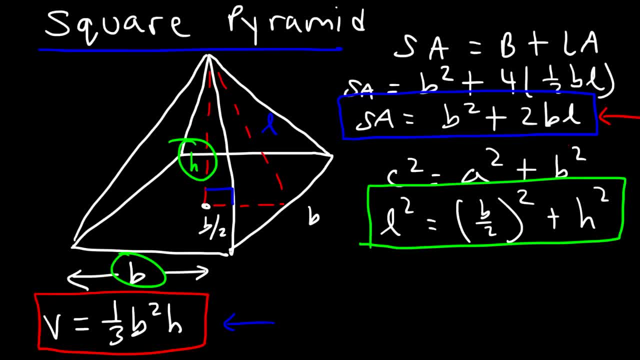 Once you have the slant height, you could plug it into this equation to calculate the surface area. So if you want to combine these two equations into one, first we need to solve for L, taking the square root of both sides, So then you'll get this equation. 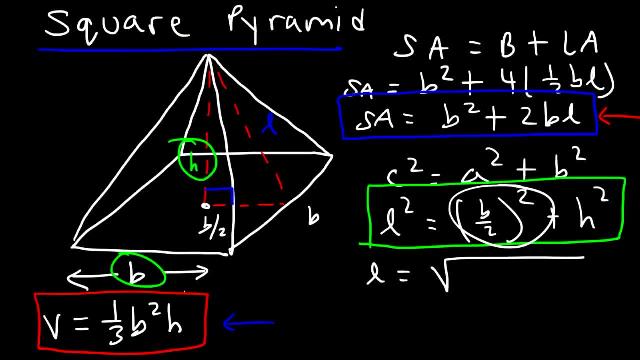 L is the square root of. this becomes B squared over four once you square it plus H squared. So I'm going to replace L with this equation And first let's make some space. So you could say: the surface area is B squared plus two, B times the square root of B squared. 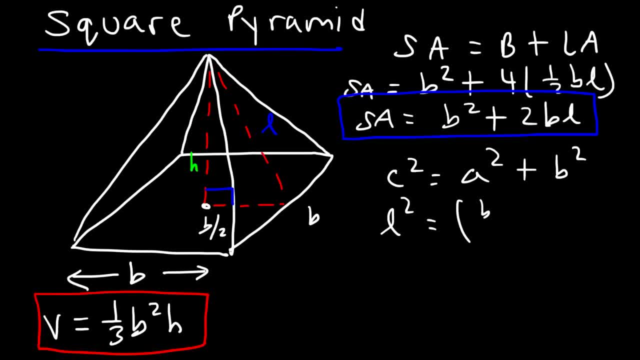 A, which we'll call B over 2.. And let's square that And then B will be H. So if you need to find the volume, you could use that equation. If you need to calculate the surface area, first you need to calculate the slant height. 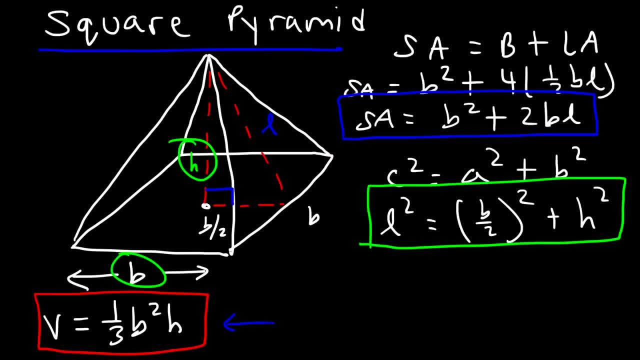 using the height of the pyramid and the base of the pyramid. Once you have the slant height, you could plug it into this equation to calculate the surface area. So if you want to combine these two equations into one, first we need to solve for L. 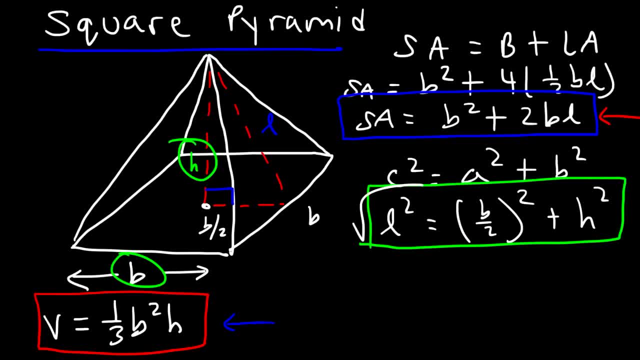 taking the square root of both sides. So then you'll get this equation: L is the square root of this becomes B squared over 4 once you square it, plus H squared. So I'm going to replace L with this equation, And first let's make some space. 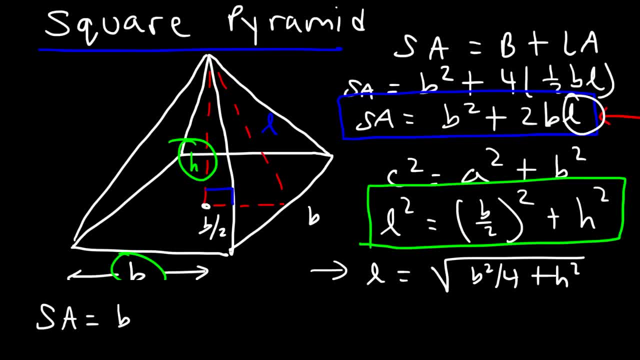 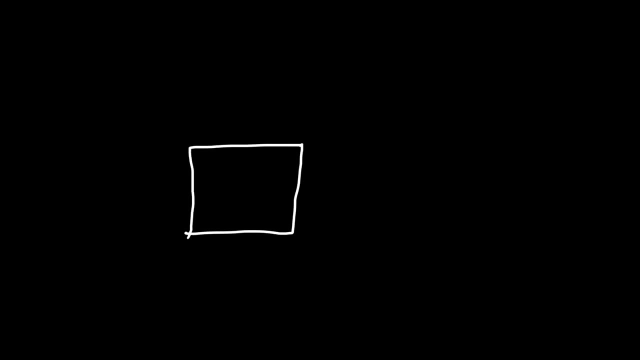 So you could say the surface area is B squared plus 2B times the square root of B squared over 4 plus H squared. So this will give you the surface area simply using the base and the height of the square pyramid. So here we have a rough sketch of a cube. 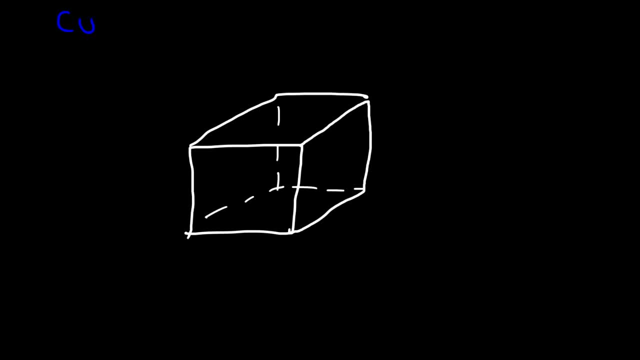 And what do you think the volume and the surface area of a cube is going to be? Well, let's say the side length is X, Just like a rectangular prism. the volume is going to be left times width, times height, So it's X times X times X. 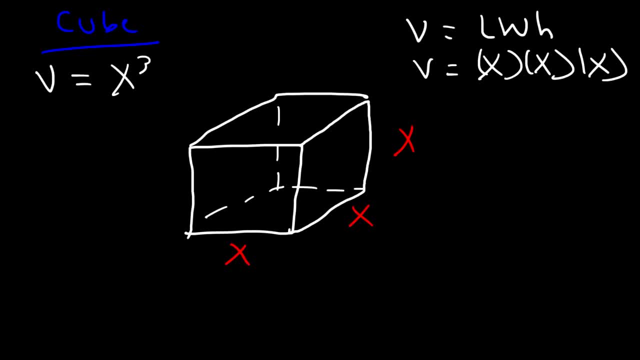 So the volume of a cube? it's X cubed Where X is the side length. Now, what about the surface area of a cube? Well, for a rectangular prism, we saw it was 2L plus 2W plus 2LH. 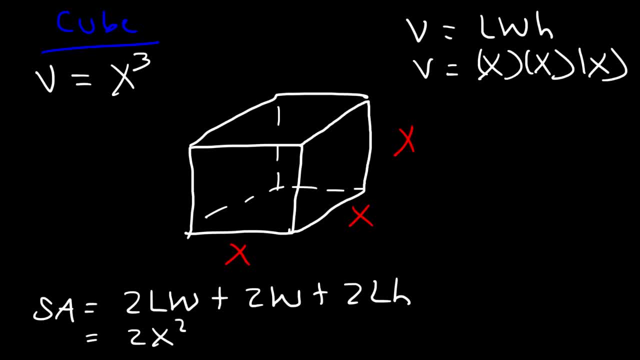 In this case it's going to be 2X squared, or like 2 times X, times X, But three times. So the surface area of a cube is 6X squared. So make sure you know these formulas. Now let's talk about the faces. 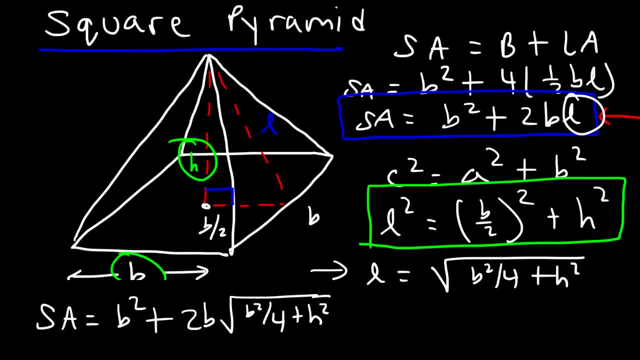 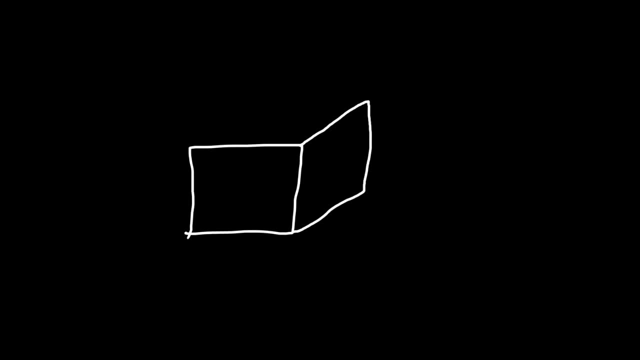 over four plus H squared. Okay, So this will give you the surface area simply using the base and the height of the square pyramid. So here we have a rough sketch of a cube. Okay, And what do you think the volume and the surface area of a cube is going to be? 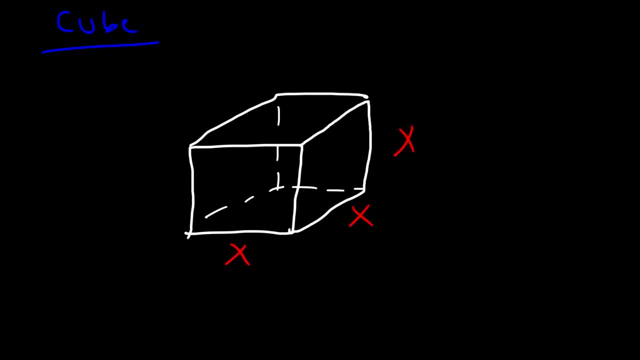 Well, let's say the side length is X, Just like a rectangular prism, the volume is going to be left times width, times height. So it's X times X times X. So the volume of a cube it's X cubed, where X is the side length. 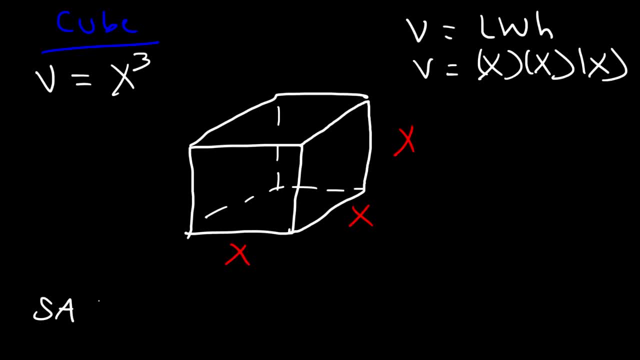 Now, what about the surface area of a cube? Well, for a rectangular prism, we saw it was 2L plus 2W plus 2LH. In this case it's going to be 2X squared, or like two times X, times X, but three times. 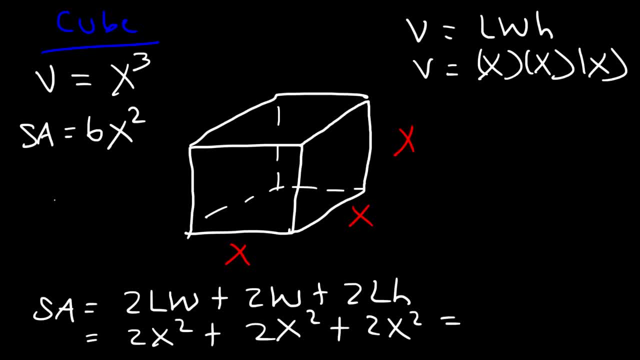 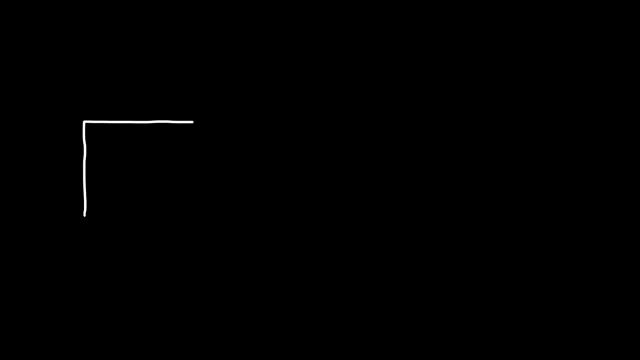 So the surface area of a cube is 6X squared, So make sure you know these formulas. Now let's talk about the faces, the edges, Okay, Okay, And the vertices of a cube. This picture was a lot better than the last one. 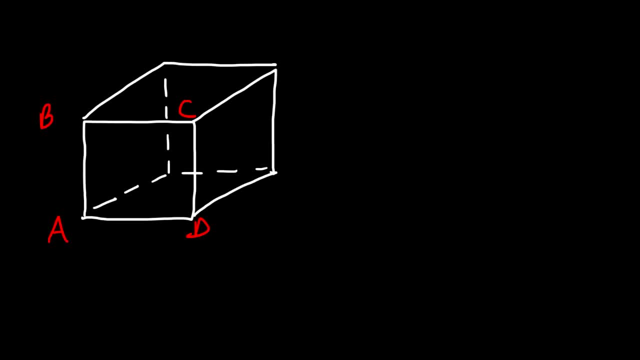 Let's call this A, B, C and D, And this is going to be E, F, G and H. So what are some of the faces of the cube? How many faces does it have? So notice that we have the face in the front. 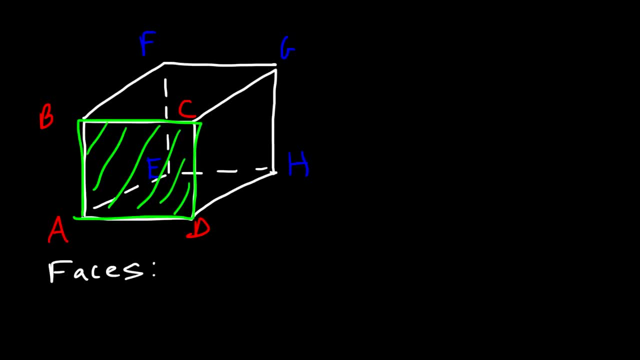 This is face A, B, C, D. Another one is the one on the side D, C, G, H. That's this one. So a face is basically a flat surface. It's two-dimensional. Okay, Now, how many faces do we have in this cube? 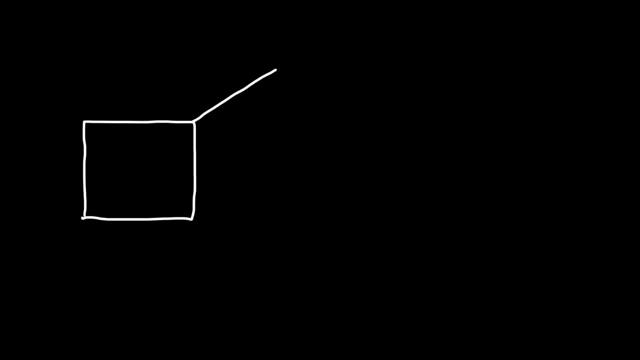 the edges and the vertices of a cube. This picture was a lot better than the last one. Let's call this A, B, C and D, And this is going to be E, F, G and H. So what are some of the faces of the cube? 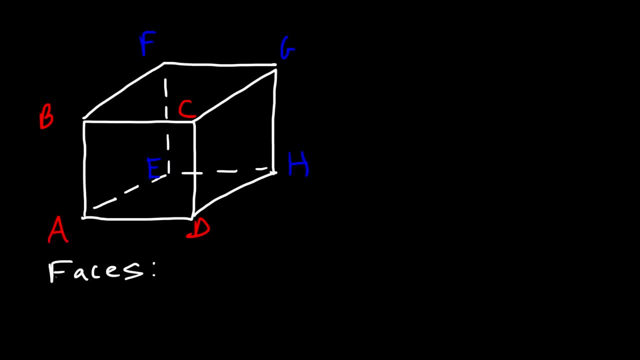 How many faces does it have? So notice that we have the face in the front. This is face A, B, C, D. Another one is the one on the side: D, C, G, H, That's this one. 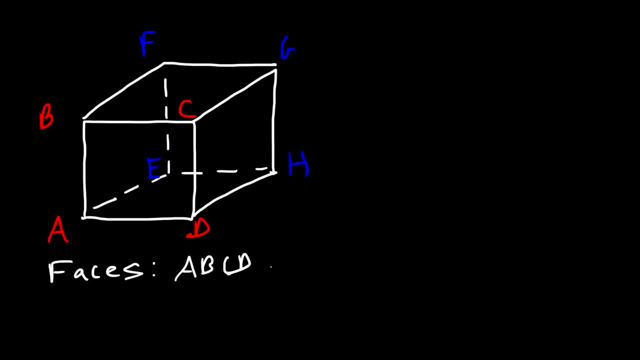 So a face is basically a flat surface. It's two-dimensional. Now, how many faces do we have in this cube? So we saw that A, B, C, D was one face. That was the one in the front We also have. 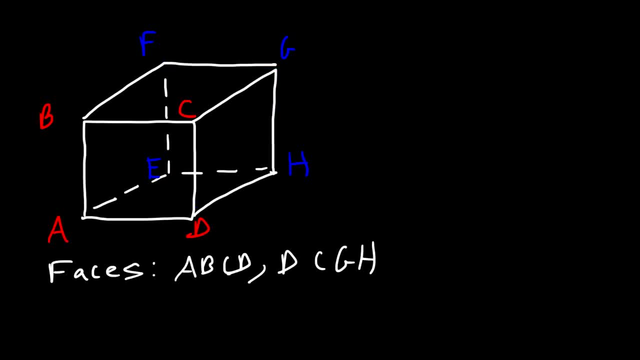 E, F, G, H in the back, That's two. On the right, we have C, D, H, G, That's three. On the left, A, B, F, E, That's four. The bottom: 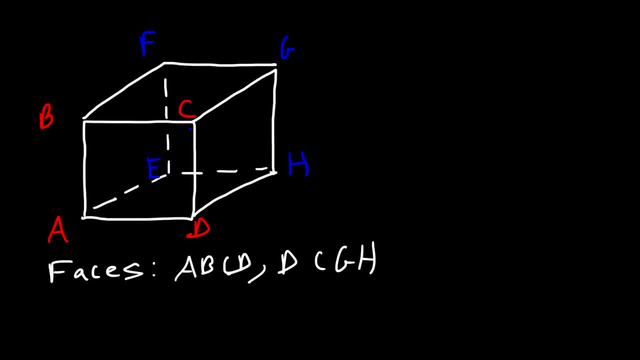 A, D, H, E, That's five, And the one on the top, B, C, G, F, That's six. So let's say that F is equal to six. Now what about the number of edges? So what are some edges in this cube? 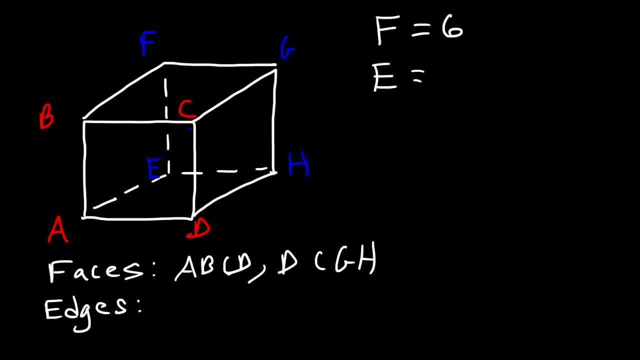 Segment A- B is an edge, So we can represent it like this: B- C is also an edge And C- D, that's an edge as well. So let's calculate the total number of edges. So A- B is one. 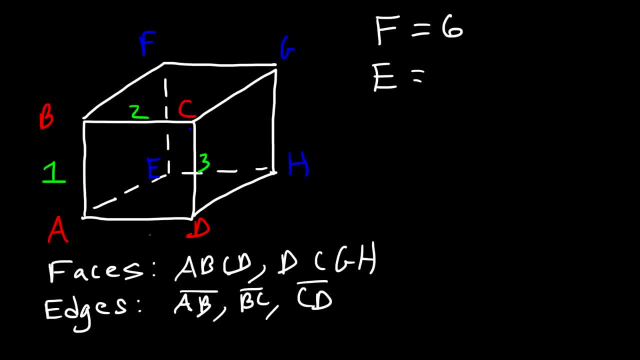 B, C is two, C, D is three. A, D is four. And then we have A E, which is five. E, H is six, D H is seven, G, H is eight. C- G is nine. 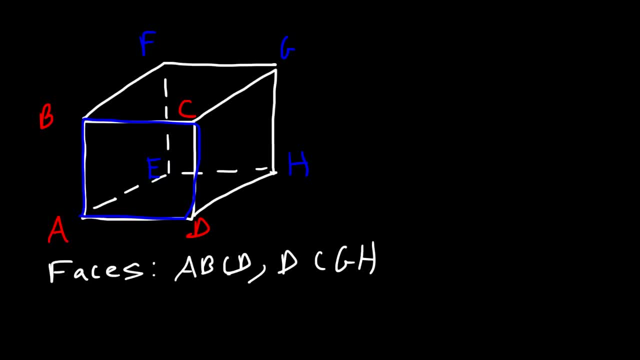 So we saw that A, B, C, D was one face, That was the one in the front. We also have E, F, G, H in the back, That's two. On the right we have C, D, H, G, That's three. 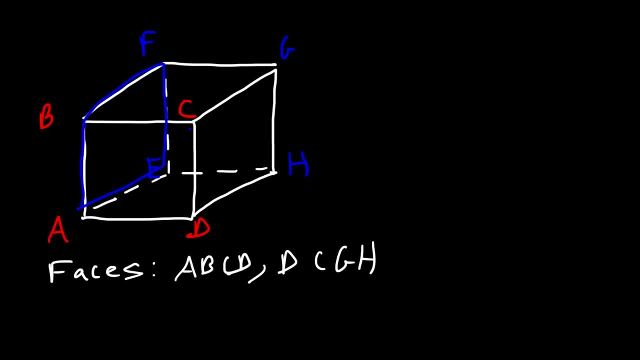 On the left, A, B, F, E. That's four. The bottom, A, D, H, E. That's five, And the one on the top, B, C, G, F, That's four. Okay, 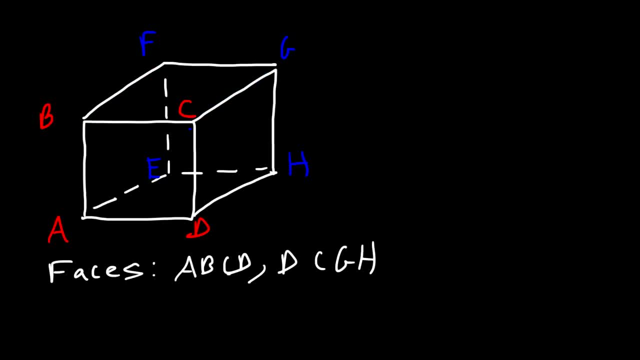 So we have A, B, C, D, G, F, That's six. So let's say that F is equal to six. Now what about the number of edges? So what are some edges in this cube Segment? AB is an edge. 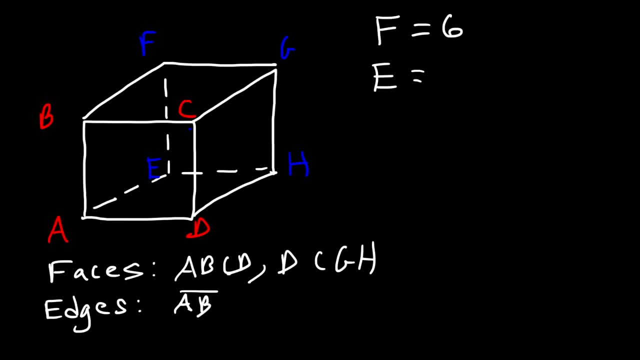 So we can represent it like this: BC is also an edge, Okay, Okay, Okay, Okay. And CD, that's an edge as well. So let's calculate the total number of edges. So AB is one, BC is two, CD is three, AD is four. 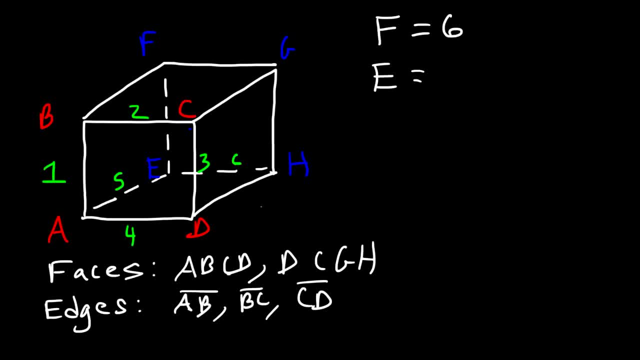 And then we have AE, which is five, EH is six, DH is seven, GH is eight, CG is nine, FG is ten, BF is 11.. And in the back we have EF, which is 12.. Okay, so a cube has 12 edges. now, what about the vertices? how many vertices to have? 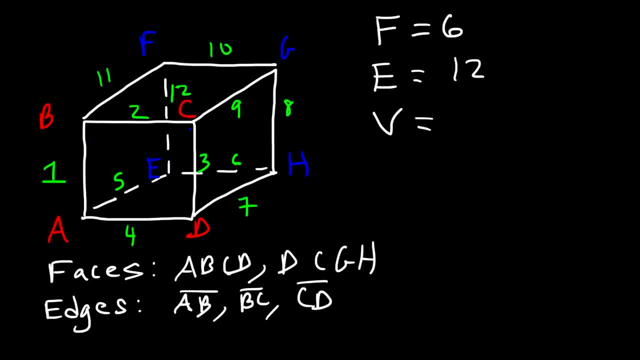 so in a cube you can identify a vertex where three edges me. so as a vertex. so it's one of the vertices. so this is one. B is another one, that's 2345678. so there's eight vertices in a cube. now you list formula tells us that the sum 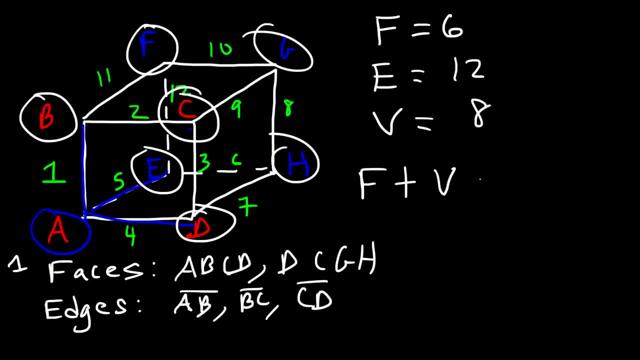 of the faces and the vertices minus the number of edges is equal to two. so in this case we have six faces, eight vertices and 12 edges. 6 plus 8 is 14. 14 minus 12 does equal 2, and so this is in harmony with Euless formula for figures. 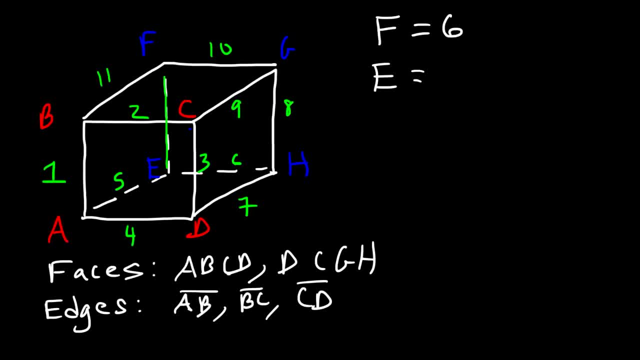 F, G is ten, B, F is eleven, And in the back we have E, F, which is twelve. So a cube has twelve edges. Now what about the vertices? How many vertices does it have? So in a cube you can identify a vertex. 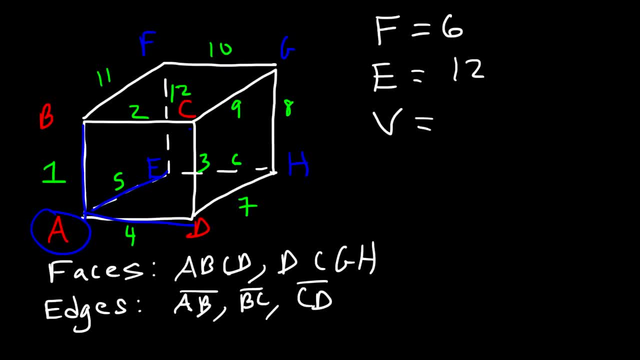 where three edges meet. So A is a vertex, So it's one of the vertices. So this is one. B is another one, That's two, three, four, five, six, seven, eight. So there's eight vertices in a cube. 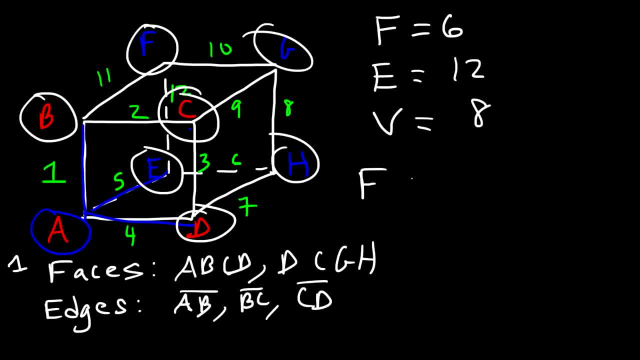 Now Euler's formula tells us that the sum of the faces and the vertices minus the number of edges is equal to two. So in this case we have six faces, eight vertices and twelve edges. Six plus eight is fourteen, Fourteen minus twelve. 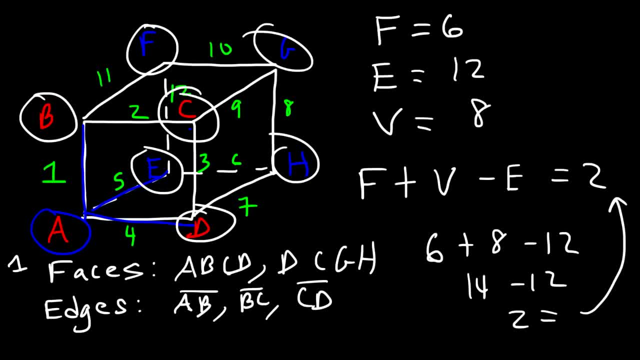 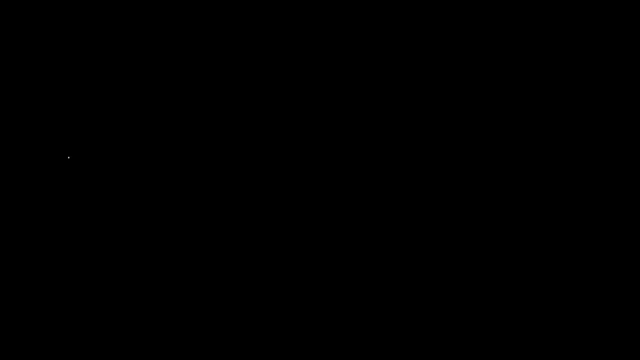 does equal two, And so this is in harmony with Euler's formula for figures like these that are just made up of faces. Now let's apply it for a triangular prism, So let's call this A, B, C, D, E and F. 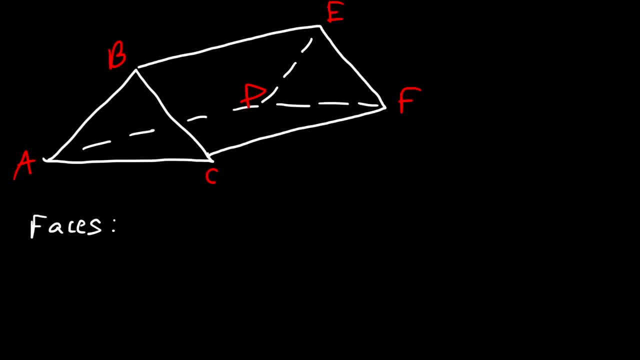 So what are some faces in this problem? So notice that A, B, C is one face of the triangle. Another face that we have is D, E, F, And also we could say B, E, F, C is a face of this triangular prism. 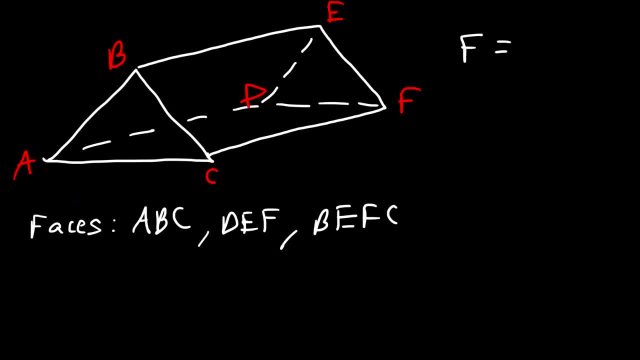 Now let's calculate the total number of faces. So the first one, as you said, was A, B, C, The second one D E, F, The third B, E, F, C. Now a fourth one is the one on the bottom. 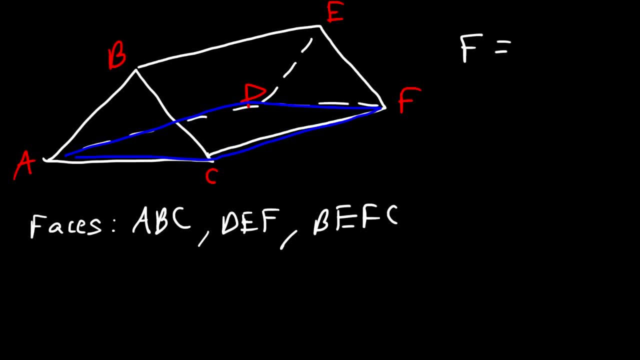 A, D, F, C, And then the one on the back left: A, B, E, D, So that's the fifth one. There's a total of five faces in this figure. Now, what about edges? Let's name some edges. 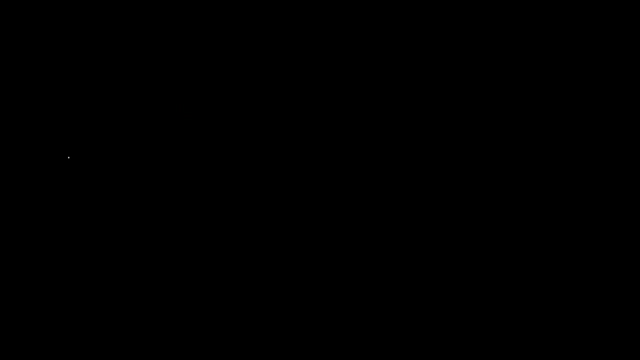 like these that are just made up of faces. now let's apply it for a triangular prism. so let's call this a, B, C, D, E and F. so what are some faces? And notice that ABC is one face of the triangle. another face that we have is: 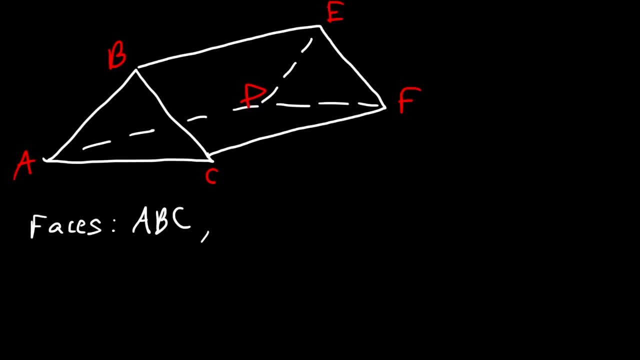 DEF, and also we could say B, E, F, C is a face of this triangular prism styling. let's calculate the total number of faces. we need to calculate organizations and individuals. one: what you see here is theнитеam of space of many cont draps, material and 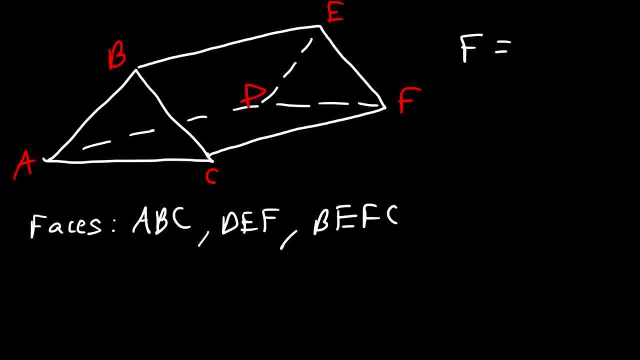 two juntos models. so if let's choose this one, rather this others word pyramid into triangular stacking bottom of the scoreboard in this problem. so notice that ABC is one face of the of faces. so the first one, as you said, was ABC, the second one DEF, the third BEFC, now a fourth. 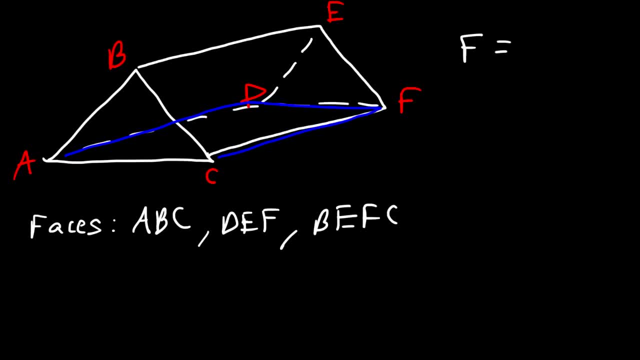 one is the one on the bottom, ADFC, and then the one on the back left, ABED, so that's the fifth one. there's a total of five faces in this figure. now what about edges? let's name some edges. so AB is an edge, we could say that BE is an edge and DF is an edge, so we can write them this way. now. 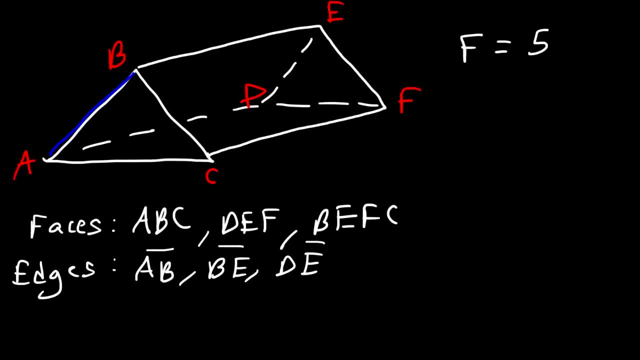 let's calculate the total number of edges. so this is one, two, three, four, five, six, seven, eight, two. let me write them. so this is: AB is one, BC is two, AC is three, DE is four, EF is five, DF is six, BE is seven, AD is eight, CF is nine. so I calculated a total of nine edges. now the vertices we just 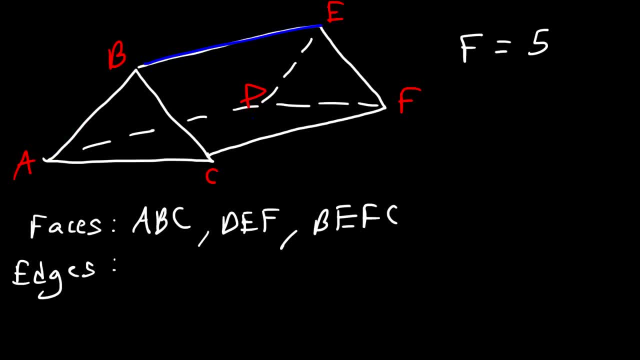 So A- B is an edge. We could say that B- E is an edge And D- F is an edge, So we can write them this way. Now let's calculate the total number of edges. So this is one, two. 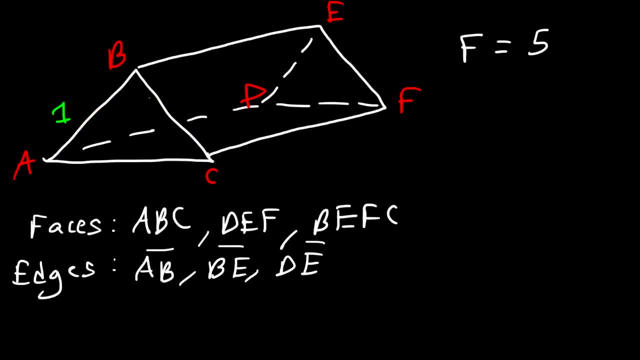 Let me write them. So this is A, B is one, B, C is two, A, C is three, D, E is four, E, F is five, D, F is six, B, E is seven. A, D is eight. 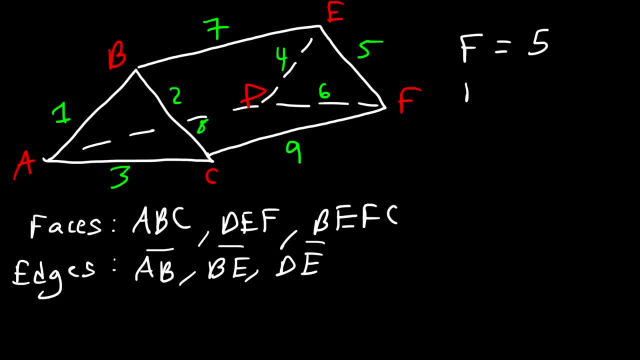 C, F is nine. So I calculated a total of nine edges. Now the vertices. we just got to count the letters, because that's where three edges will meet. So this is one, two, three, four, five, six. So I counted six vertices. 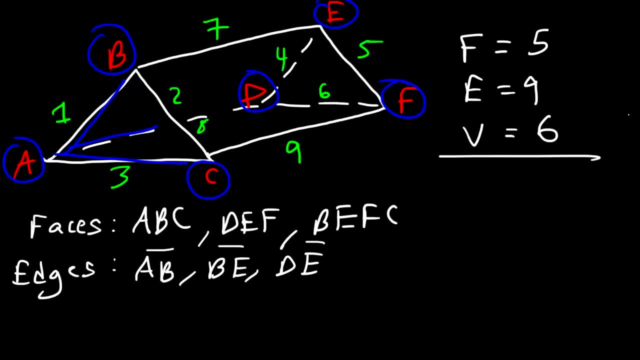 Now let's use Euler's formula to confirm that this is equal to two. So the faces plus the vertices, minus the edge lengths, has to equal two. So we have five faces, six vertices and nine edges. Five plus six is eleven. Eleven minus nine is two. 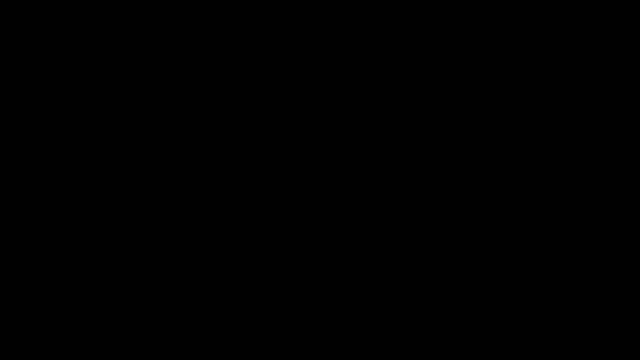 So this is in harmony with Euler's formula. Now let's go over one more example, And so that is the square base pyramid. So let's call this A, B, C, D and E. So let's calculate the number of faces. 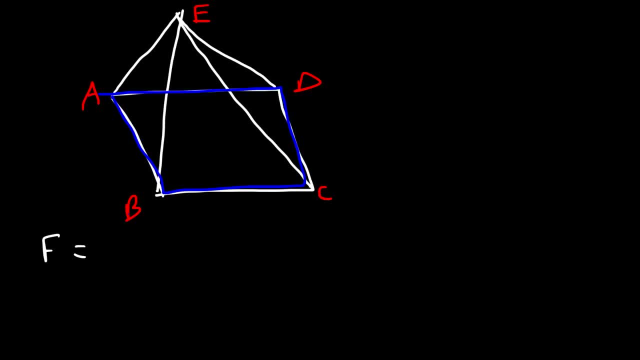 So we have face A, B, C, D. That's the base of the pyramid. Another face is A, E, B. That's two, And then E B, C is another one. So that's three, And then E C, D. 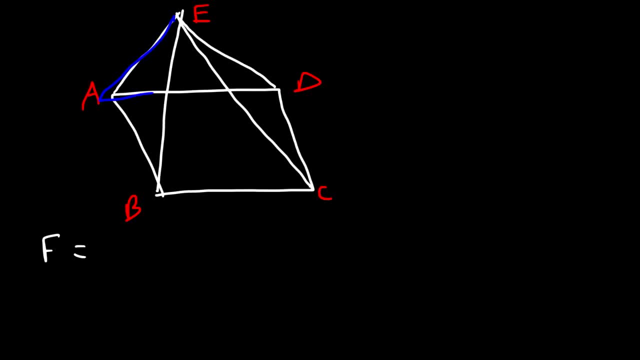 That's four, And then the one in the back: E, A, D, That's five. So there are five faces in this figure. Now the number of vertices are the letters A, B, C, D, E. So there's five vertices. 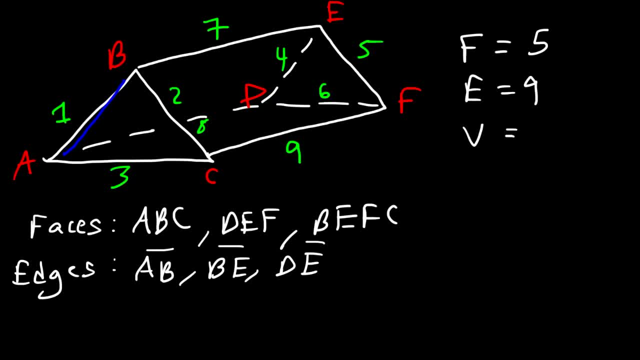 gotta count the letters, because that's where three edges will meet. so is 1, 2, 3,, 4, 5, 6.. So I counted six vertices. Now let's use Euler's formula to confirm that this is equal to 2.. So the faces plus the vertices, minus the edge lengths has to equal. 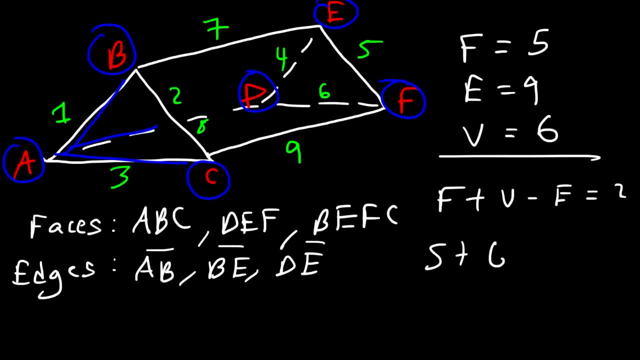 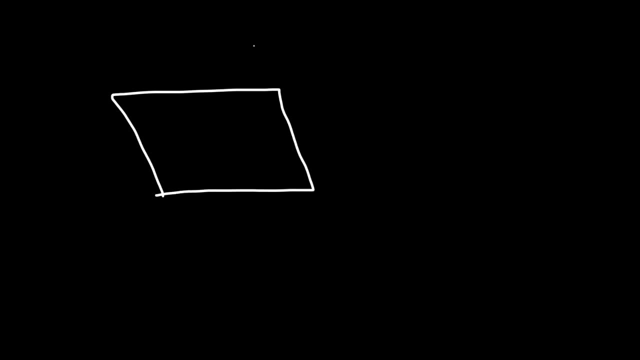 2.. So we have five faces, six vertices and nine edges. 5 plus 6 is 11.. 11 minus 9 is 2.. So this is in harmony with Euler's formula. Now let's go over one more example, And so: 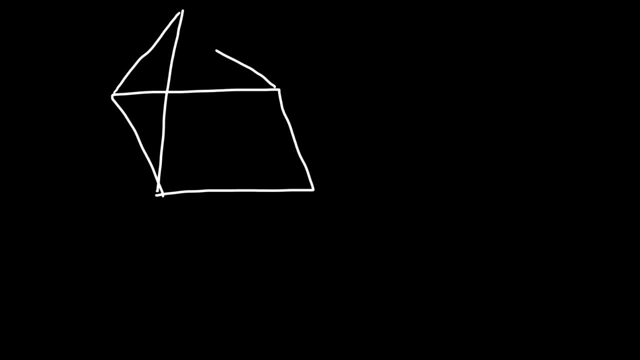 that is the square base pyramid. So let's call this A, B, C, D and E. So let's calculate the number of faces. So let's calculate the number of faces. So let's calculate the number of faces, So we have face A, B, C, D. That's the base of the pyramid. Another face is A, E, B, That's. 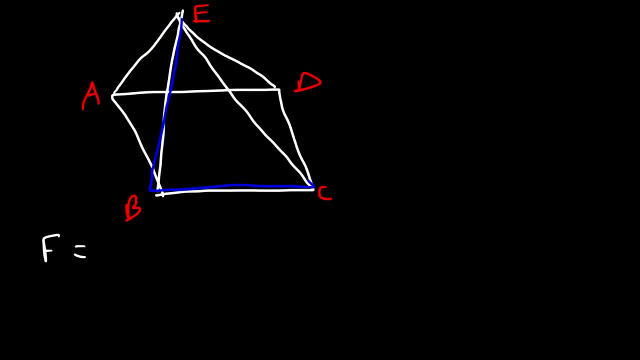 2.. And then E B, C is another one, So that's 3.. And then E C, D, That's 4.. And then the one in the back, E A, D, That's 5.. So there are five faces in this figure. Now the number: 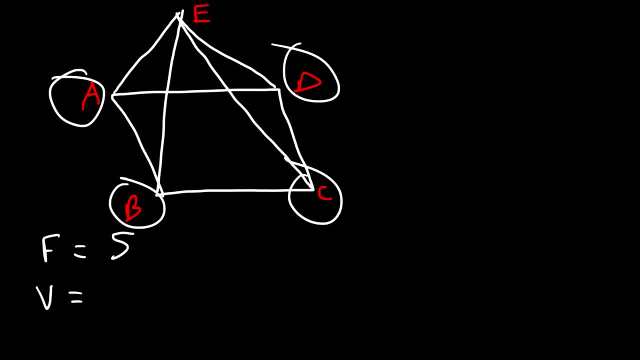 of vertices is D, E, and this is where you have the edges. so there are 5 vertices. now Let's multiply the edges. So we have edge AB, That's 1.. And then there's AE, That's another one, And then, once again, this one is for the comigo factors in, And that's 1,, 2,, 3,. and 4.. And that's the second. So this is counterpoint: 1, 2,, 1, 2.. Then we have thePOEST and on top of that is the vertex. When we put the reference to 0,, 2,, 3,, 0, 5,, we get E. B, C, D and E, so there's 5 vertices. Now how many edges are there? So we have edge AB, That's 1.. And the characterekt room, other 1, is BF, that's Donkey It'sadeaho. 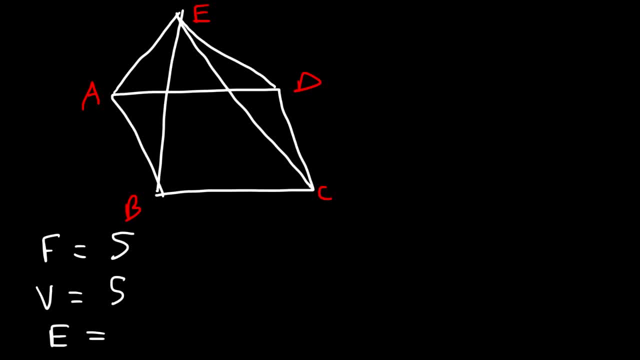 Now how many edges are there? So we have edge A, B, That's one. A E, That's another one. B E, That's number three. Let's use a different color: B C is four, E C is five. 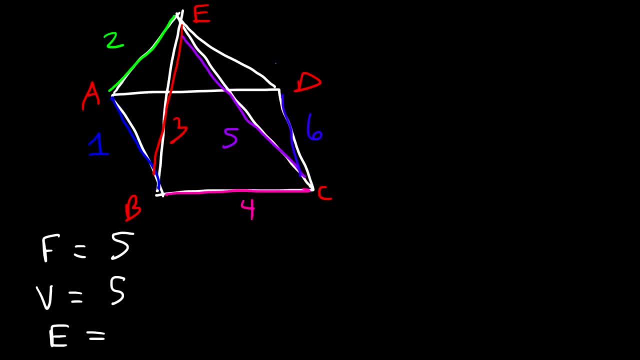 D, C is six, A, D is seven And then E, D is eight. So I got a total of eight edges. So the faces end up and the vertices minus the edges has to equal two. So F is five, V is five. 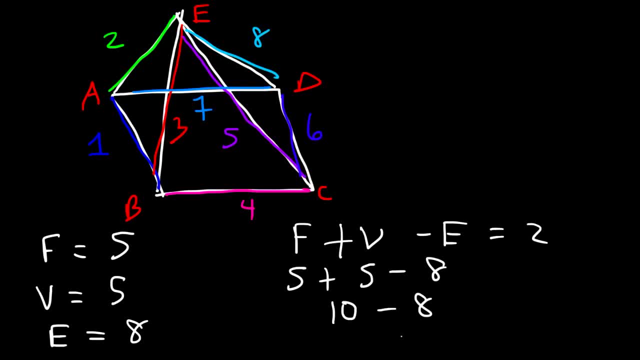 And E is eight. Five plus five is ten. Ten minus eight is two, So this is another figure that works in harmony with Euler's formula, And so that's it for this video. Hopefully it gave you a good introduction into 3D shapes such as. 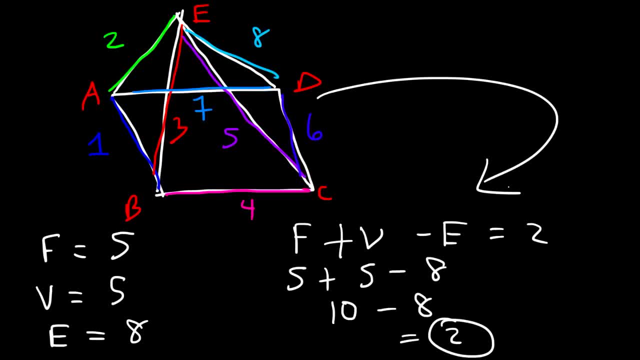 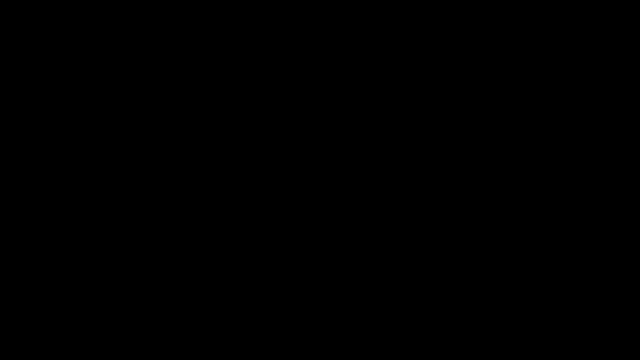 spheres, cylinders, cones, rectangular prisms, square-based pyramids and things like that. So thanks for watching. Okay. so this video is not for those of you who want to become a hacker in the next two to three weeks. This video is for somebody who actually wants to learn how to become an ethical hacker, whether it is bug bounty hunter or a penetration tester. So I keep seeing videos that say: 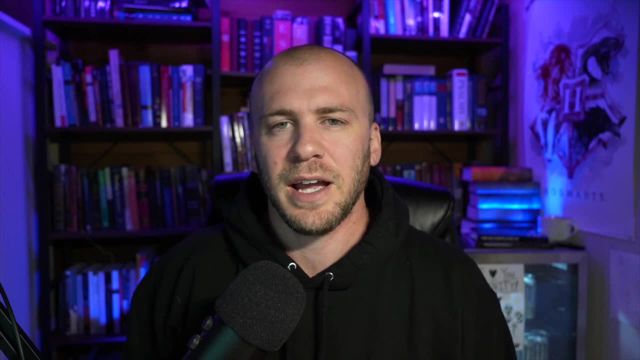 everything you need to know in order to become a bug bounty hunter or an ethical hacker, And in these videos, all they do is pull up a PowerPoint or just list off five things, such as learn Linux, learn Windows, learn some privilege escalation and maybe five of the 10 OWASP top 10 and boom. 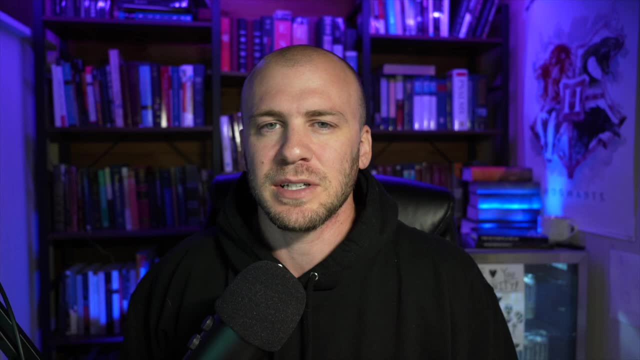 you're ready to go, And I can say that I am guilty of doing some of these similar things- maybe not to the same level- And they've just started to annoy me. So I decided to make a video that doesn't just say you need to go and learn these things, but actually show you where you're. 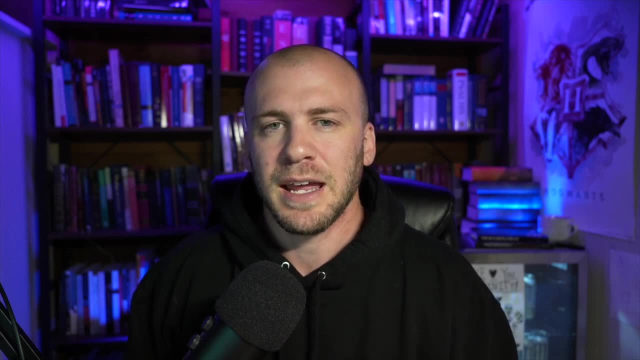 going to go to learn the information that you need, and the best places that will be free and those that will cost as little money as possible. We're all familiar with those tutorials that are really worthless and look something like this: Okay, in order to become a hacker, all you need